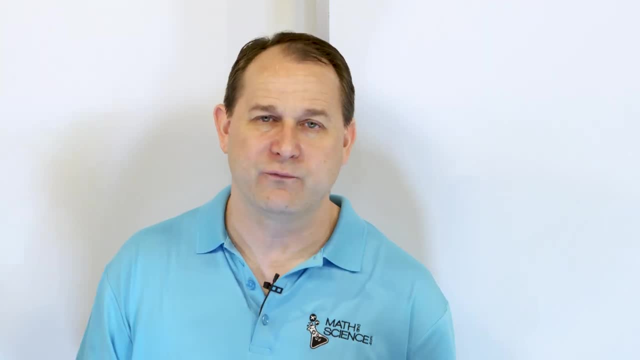 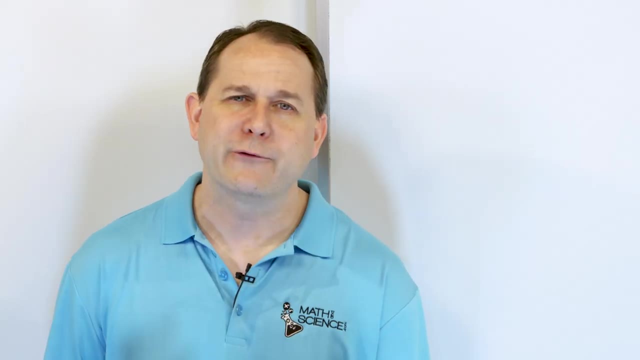 to do is read the definition of a reference angle. I don't want to write it down because it's very simple to understand and it will just take too long to write it. But we'll talk about it and we'll do a ton of problems. So the reference angle is called theta prime, So usually we use the. 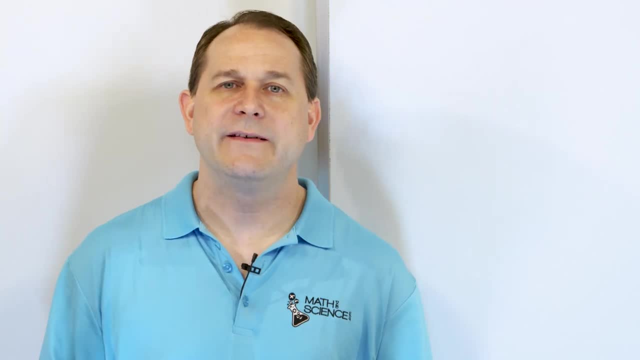 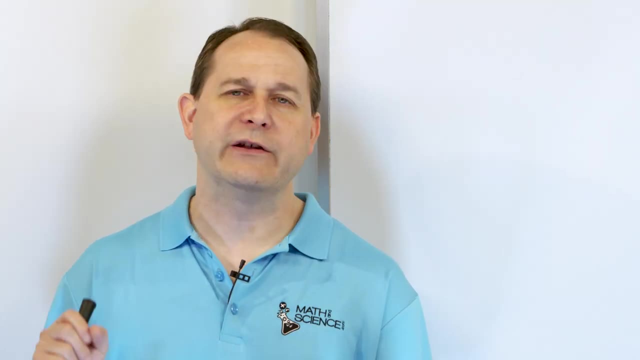 Greek letter theta to represent an angle. Theta prime is a reference angle. It's related to theta, but it's a different angle. It's called theta prime. It's the smallest acute angle between the terminal side of an angle and the x-axis, and 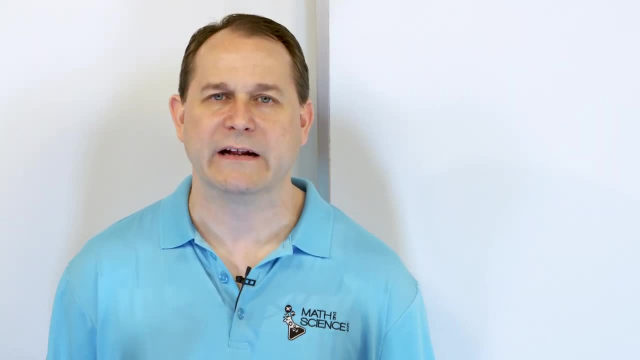 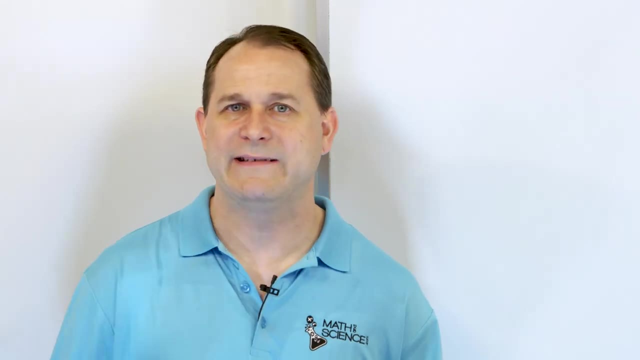 is denoted theta prime. Theta prime is always positive and it's always acute. Now, if you're like me, you read this the first time. it makes no sense, So what I'll do is I'll show you on diagrams exactly what it is. It's very simple. Read it one more time. A reference angle- theta. 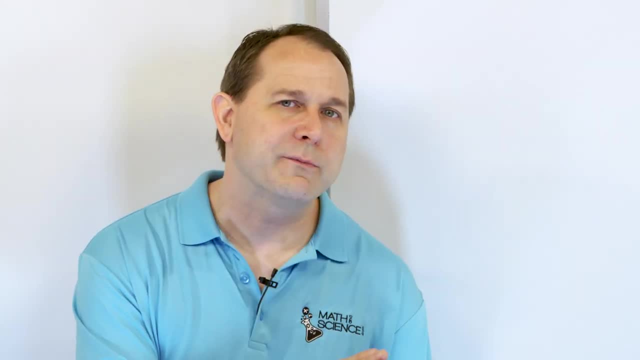 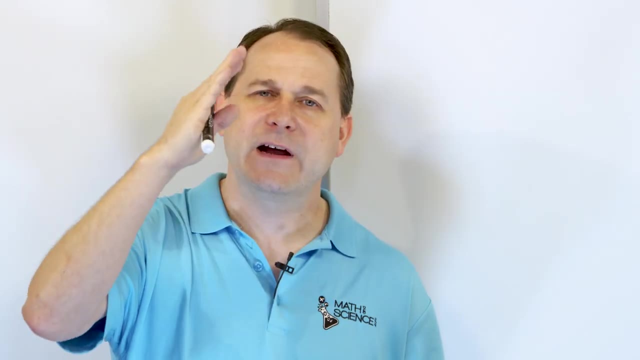 prime is the smallest acute angle between the terminal side of an angle and the x-axis. So it's basically what you want to do is look at the angle, no matter where it is, and figure out how many degrees exist between that angle and the x-axis anywhere around the unit circle. You're always 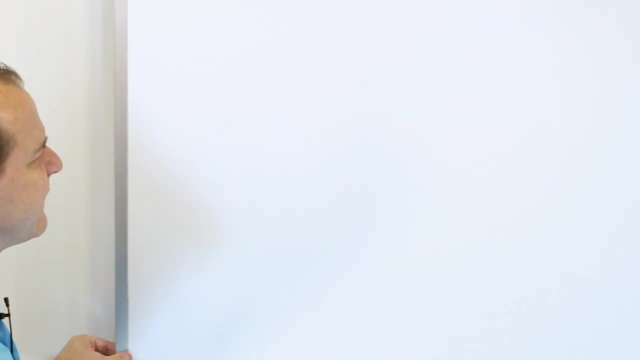 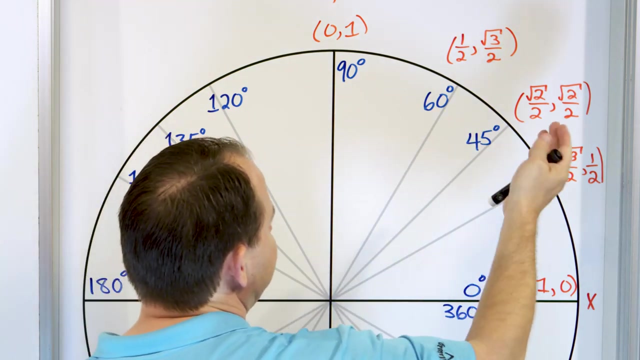 going to get a positive number for the reference angle, All right. so let's talk about it before we solve some problems. Just talk through it a little bit. Reference angle: smallest angle between the terminal side of an angle and the x-axis. So let's say you had a 30 degree angle. This was 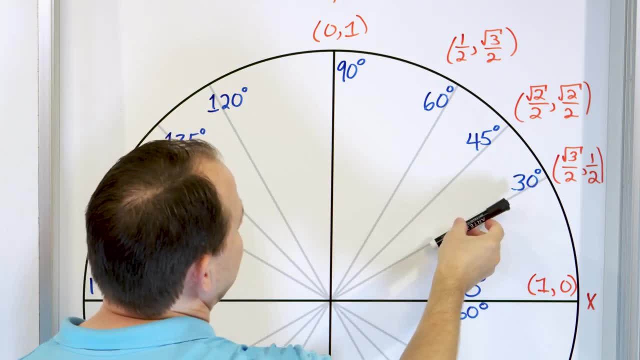 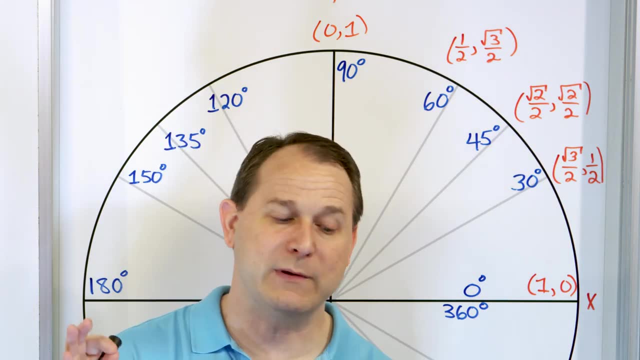 theta. And I ask you: what is theta prime, the reference angle? And you're going to say: well, in this case this angle is 30 degrees up, as measured from the x-axis. So the definition says it's the smallest acute angle between the terminal side. Remember, this is the terminal side, This is 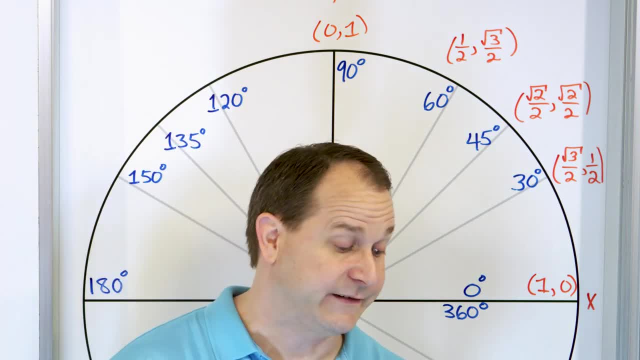 it right here, The smallest acute angle between that and the x-axis. So if the angle is really 30 degrees theta, then theta prime, which is the reference angle, is also 30 degrees, because it's just the angle to the x-axis, That's all it is. What about 45 degrees? If this is the angle, 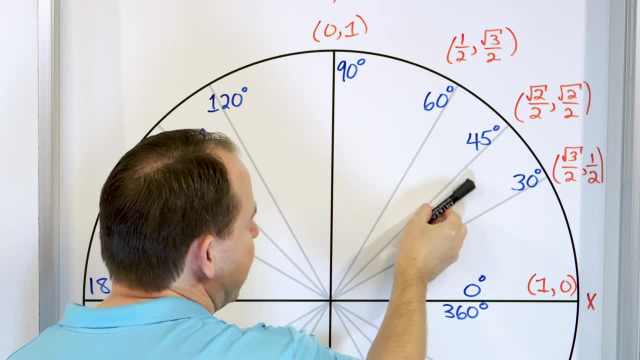 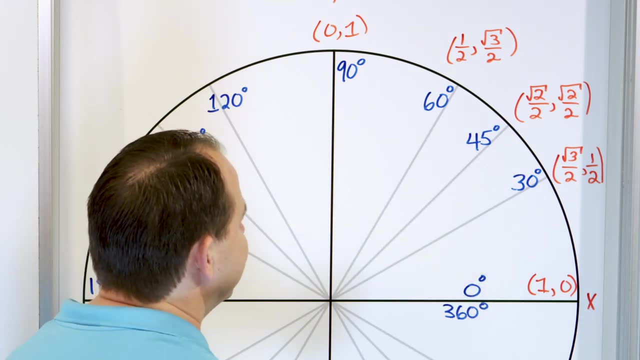 theta. what is theta prime? Well, theta prime is the same thing. It's the same angle to the x-axis. It's the 45 degrees between it and the x-axis. 60 degrees- same thing. The reference angle here is between that and the x-axis. Now let's go way over. let's say here to 135 degrees. You all know. 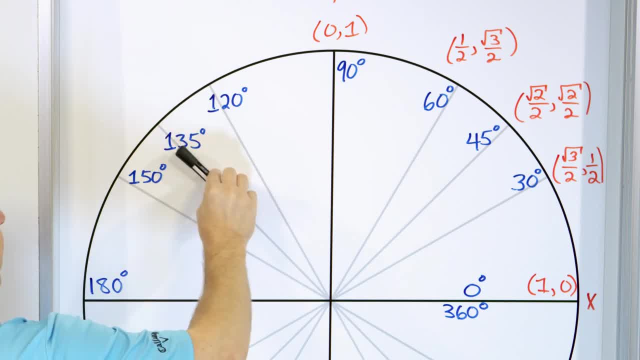 that this is like the mirror image of the 45 degree line over here. right, So what is the angle here? theta, The angle is measured all the way to. here is what it says: 135 degrees. Now what if I ask you what is the reference angle over there? The reference angle, remember, is the smallest. 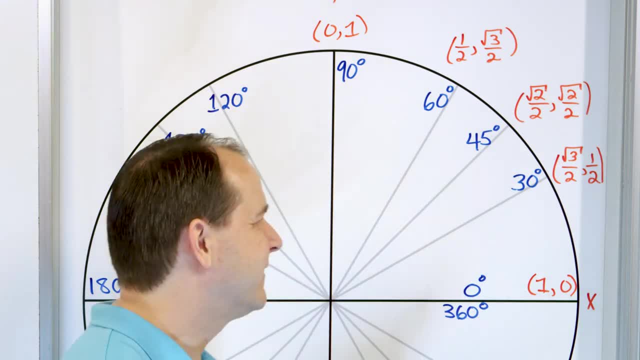 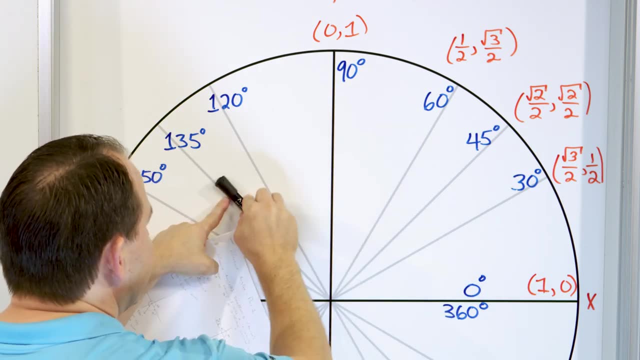 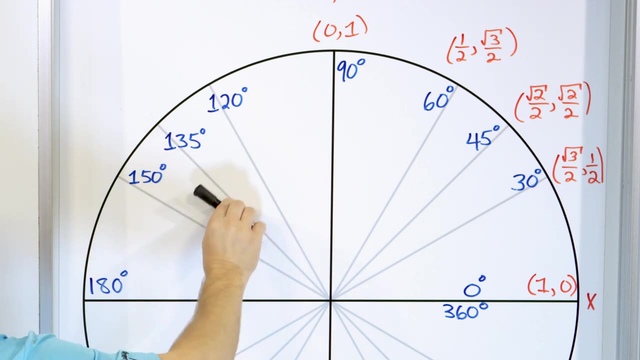 angle which is acute between the terminal side and the x-axis. So here's the angle: 135.. The angle from here to this x-axis over here is 135 degrees. But the reference angle is asking me what is the smallest angle, the acute angle, between this and the nearest x-axis? This over here is the negative. 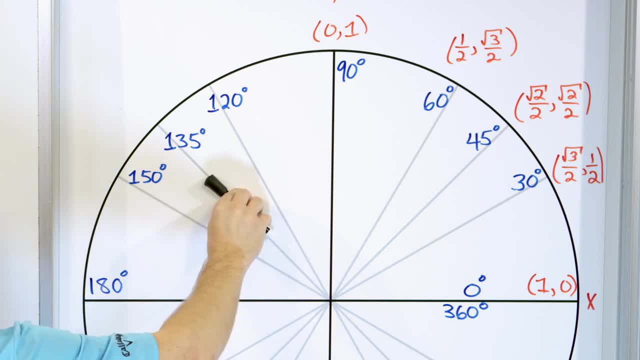 x-axis. It is the nearest x-axis from it And so the terminal angle- I'm sorry- the reference angle will be 45 degrees. If you get a protractor out and stick it here and measure this angle from here to here it's going to be 45 degrees. So if you get a protractor out and stick it here and measure, 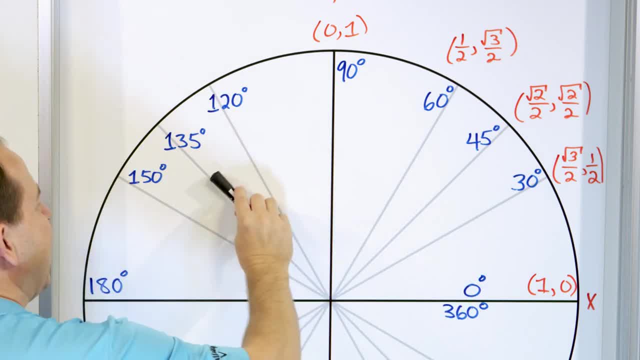 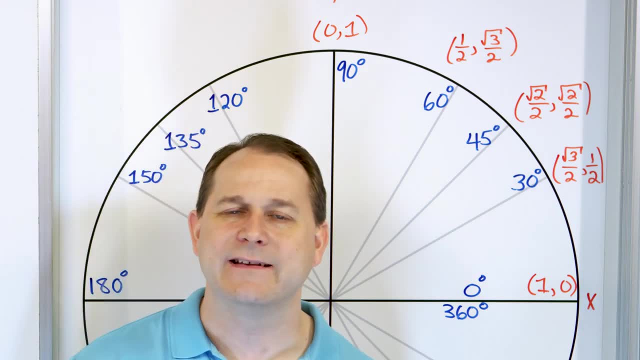 this angle from here to here you will measure 45 degrees. So here the angle theta is 135, but the reference angle here is 45. It's just the angle from wherever you're at to the x-axis. Take away any signs, no negative numbers, just what is the angle between that place where you're at, on the 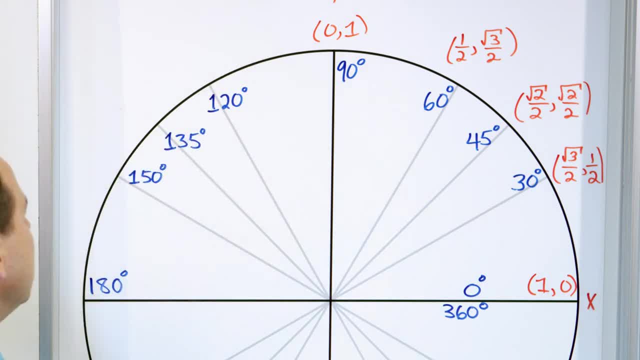 unit circle and the nearest x-axis that you have access to. So let's just go through rapid fire, right? We're just going to go real fast around the unit circle and then we'll do a bunch of problems to write them down. What's the reference angle here? This is what the reference angle is. 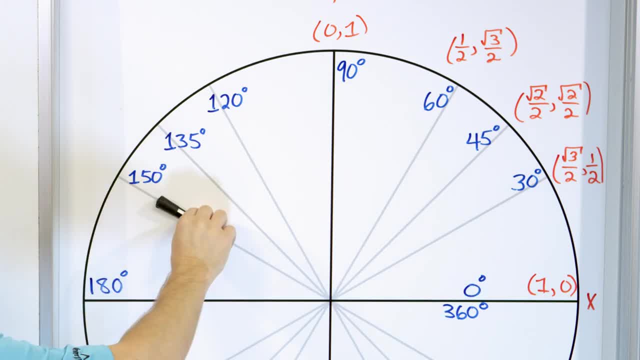 150 degrees as measured from here. The reference angle is the smallest angle between this and the x-axis, That's 30 degrees. So the reference angle between here and here is 30 degrees. What is the reference angle of 120?? 120 degrees is here. The reference angle here is: this is 60. 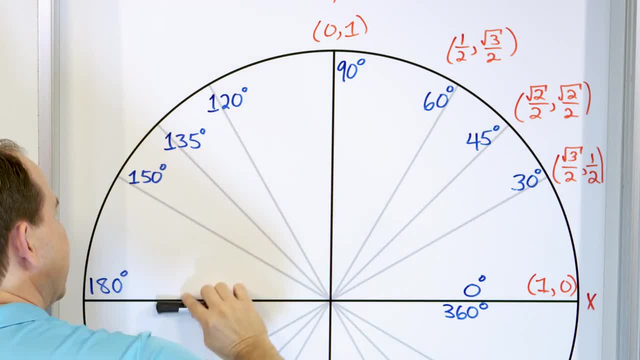 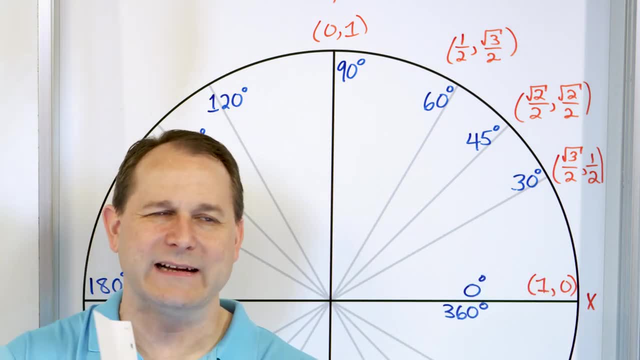 degrees. You can see from symmetry that this is kind of like the 60 degree line over here and this is the 45 degree over here and this is the 30 degree. Of course it's on the other side, so you could kind of say it's negative, but for reference angles we don't care about signs. I 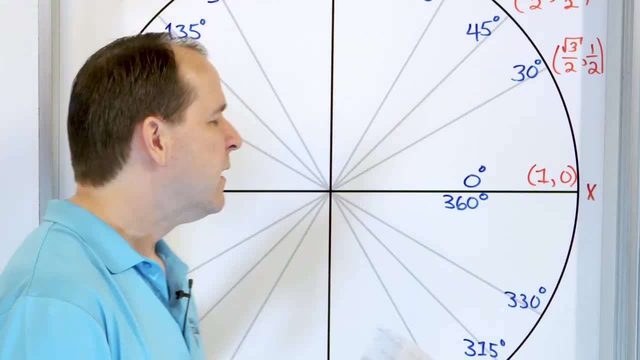 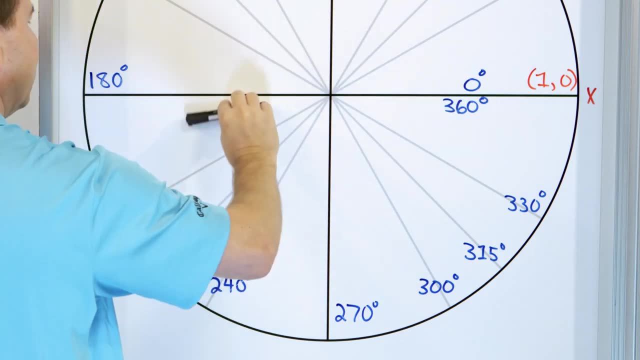 want to know If I get a protractor out, how many degrees is it? Now, if you go down here, it's the same thing. This angle is 210 degrees. That means the angle all the way measured from here is 210.. 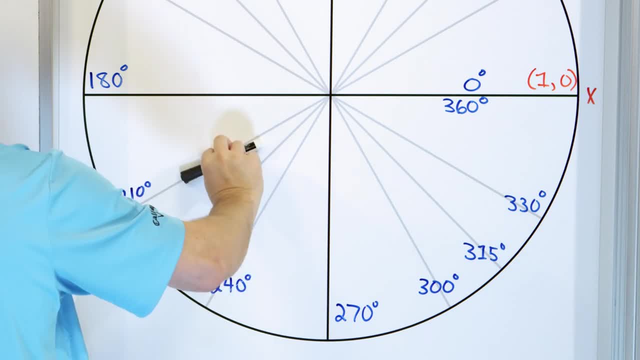 But the reference angle, theta prime, is just the angle to the nearest x-axis. This is 30 degrees, So the reference angle is 30 degrees. The reference angle between this and the axis is 45 degrees. The reference angle between 240 over here. 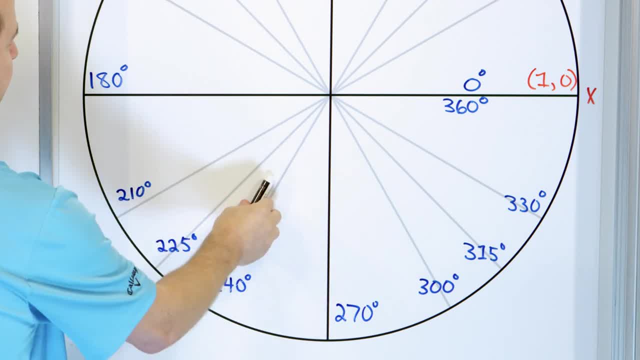 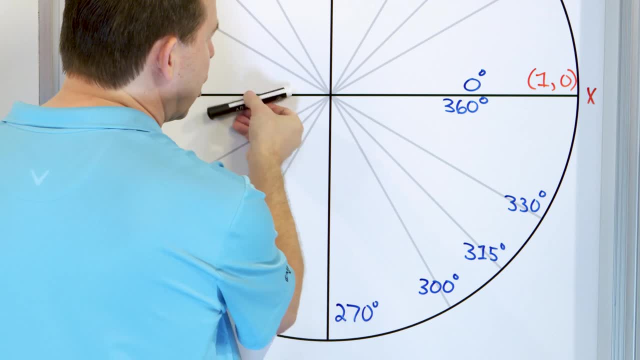 is the nearest x-axis, which is 240 degrees, I'm sorry, which is 60 degrees. You could say the reference angle here is 90 degrees. When you get over here, the reference angle no longer goes to this axis. It goes to the nearest x-axis because it 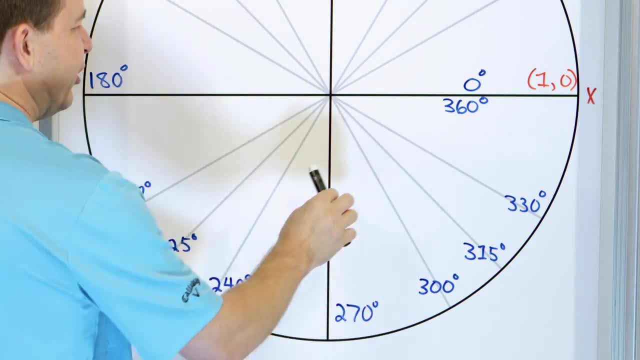 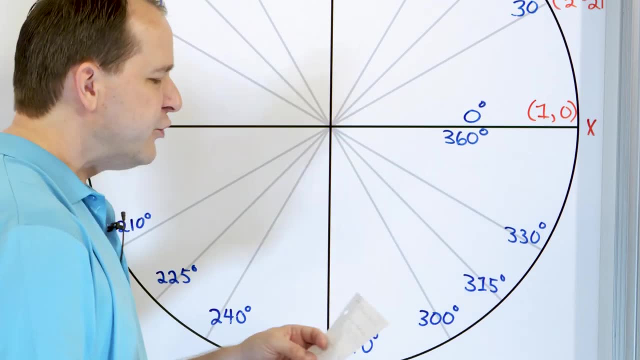 has to be an acute angle. The reference angle is the smallest angle which is acute. So from this to the nearest axis is 60 degrees, Then this will be 45 degrees, Then this will be 30 degrees. You might say: why do we care about reference angles? 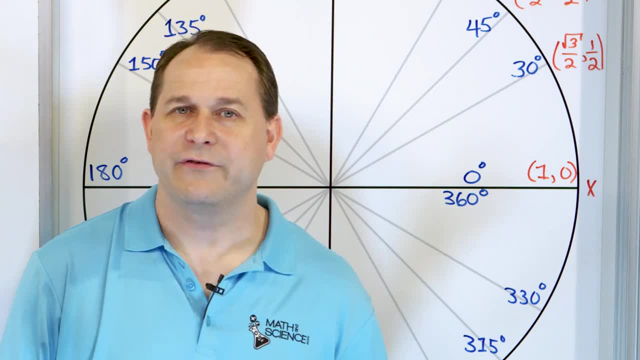 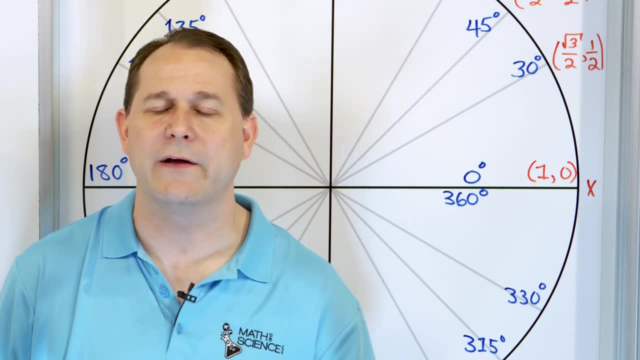 Because don't we care about the actual position of the angle? Well, the answer is kind of yes, but also reference angles help us very quickly calculate the sine and the cosine of numbers anywhere around the unit circle. I'm actually going to get to that a little bit later. 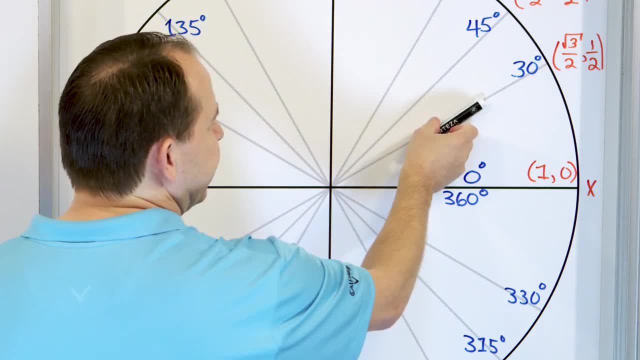 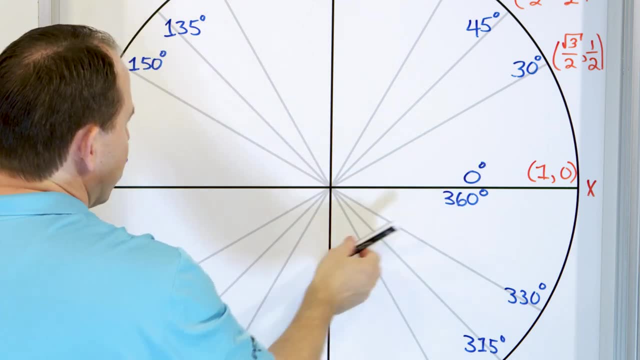 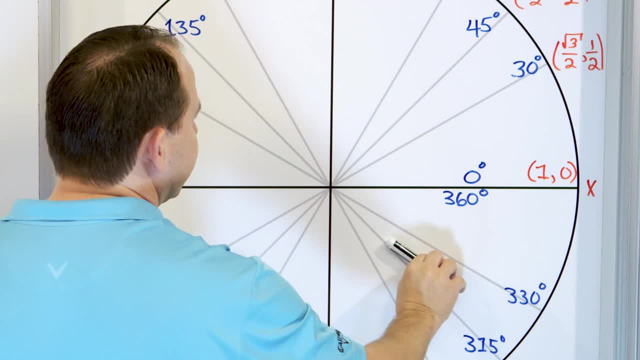 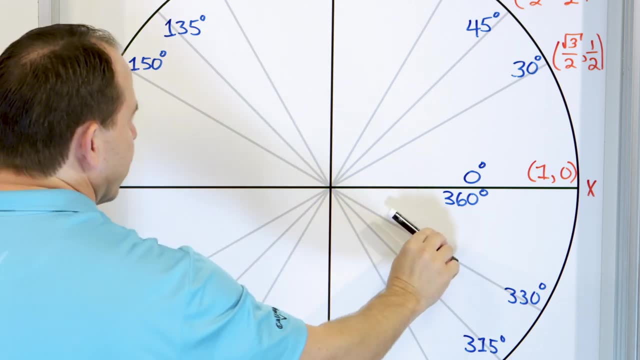 Reference angle of this: 45 degrees. Reference angle of this: 45 degrees. Reference here: 45.. Reference here: 45.. I can go on and on. Reference here: 60.. Reference here: 60. Reference here. 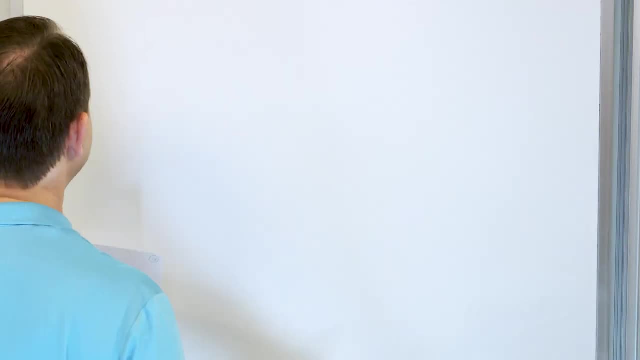 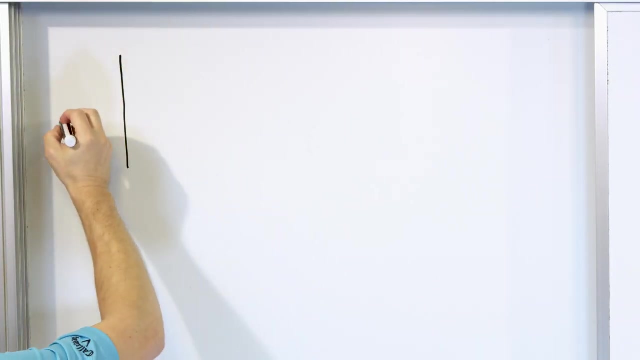 60,. it's just the smallest angle to the nearest x-axis that you have access to. Now, having talked through it, these problems should be quite simple, But I still want to do them because we need to write something down. So if we have an xy-axis here and I tell you 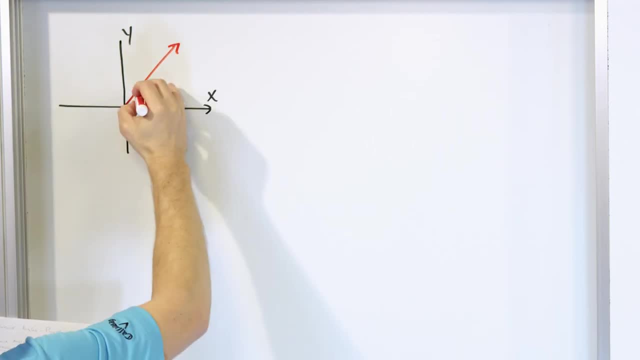 here is an angle like this And I say, hey, this angle is theta, And I tell you, theta is 60 degrees. I'm going to ask you a question: what is theta prime? equal Theta prime is the reference angle. 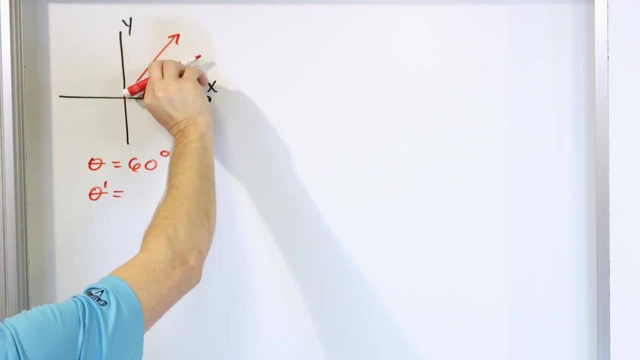 So you just look up here and say, well, if this is 60 degrees, then the distance between this to the nearest axis is actually 60 degrees. So in this case, in quadrant 1, the reference angle is the same as the actual measurement. 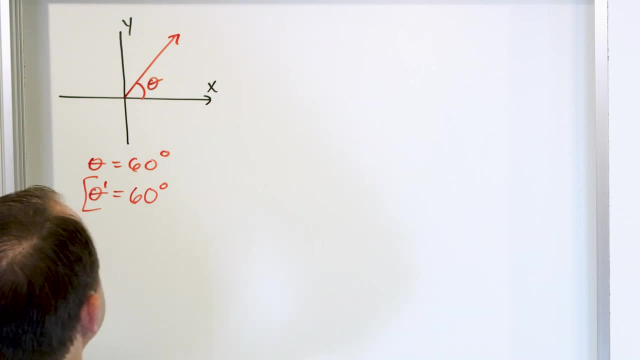 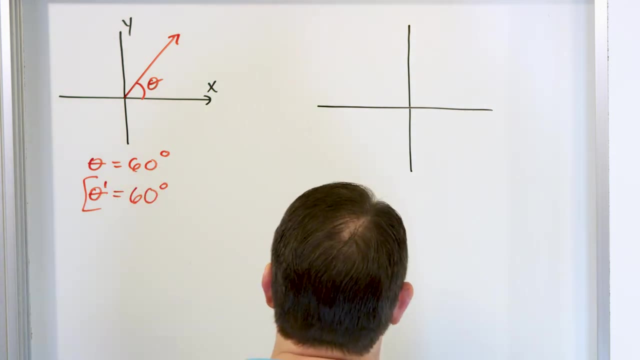 of the regular angle in quadrant 1.. In the other quadrants then they can be different. What if I have over here, switch things up again a little bit, use purple. Let's say, over here I have an angle, And actually just for completeness, 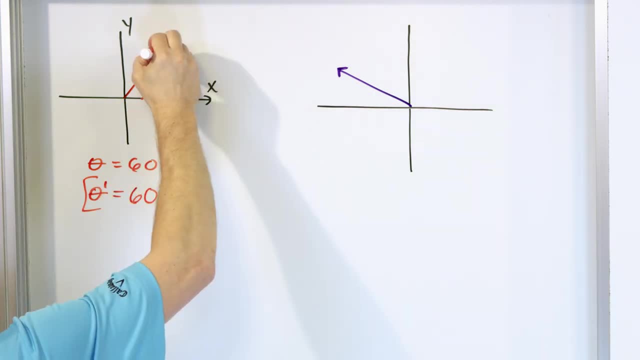 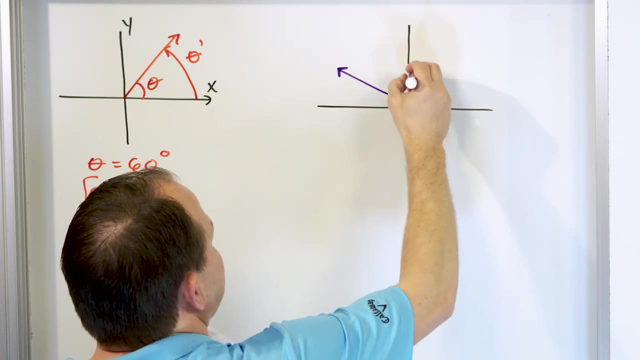 I'm going to say, since 60 degrees is the angle, then theta prime is also measured here, which is- I'll label it on the diagram. Now, over here, let's say that the angle is measured again, as it always is, from here. 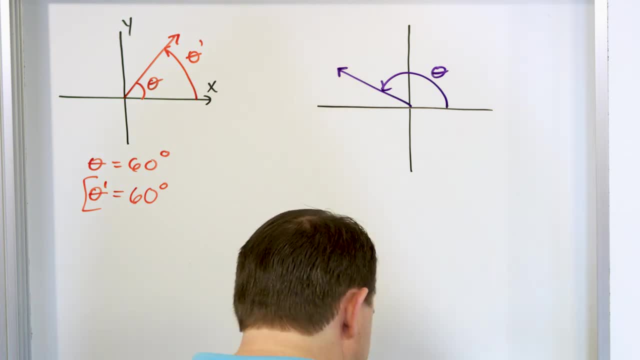 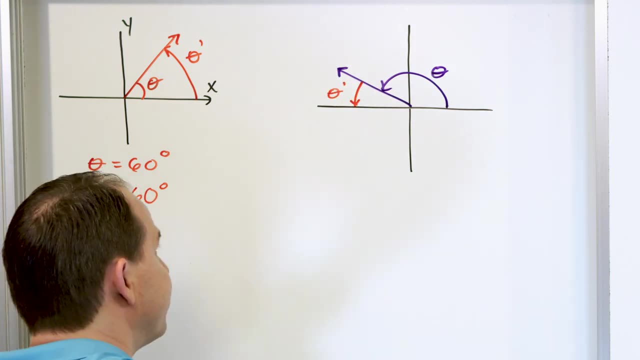 This is angle theta And theta prime is measured from this position to the nearest x-axis. theta prime, just like this. So what would if I give you that theta is 150 degrees? how do you find theta prime? Well, we did it on the diagram over there. 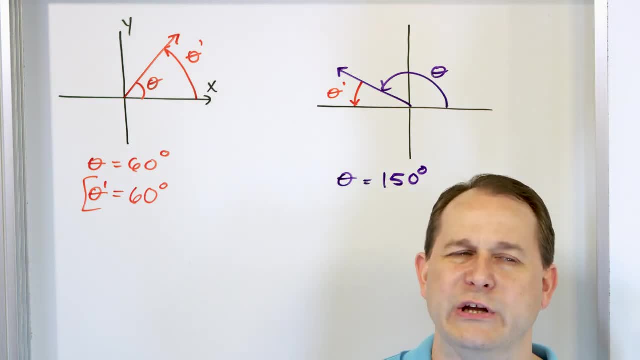 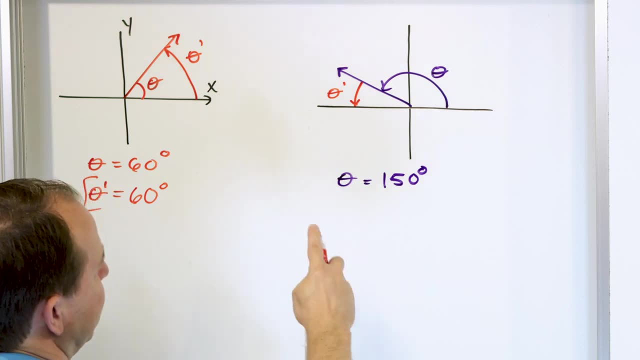 because we kind of are familiar with those diagonal lines. We know how far away they are from the positive x-axis, So we kind of know on the other side how far away they are as well. But the real way to do it is, you would say well. 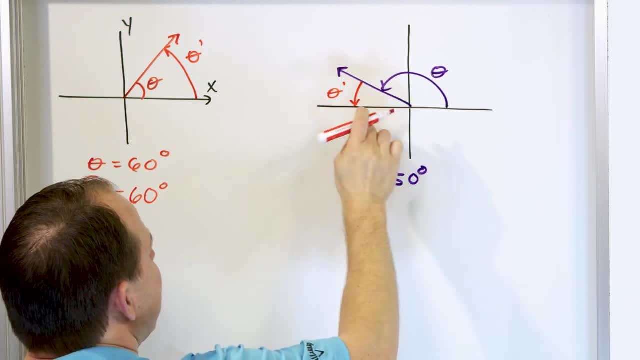 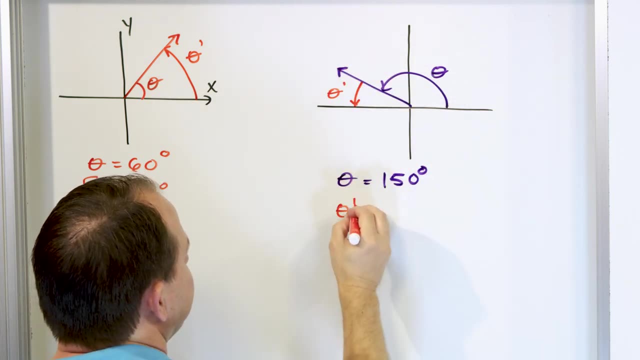 we know this black line is 180 as measured from this direction, And we know that this purple angle is 150.. So really, theta prime should be 180.. And that's exactly what you're doing in your mind When we go over there and we look at it. 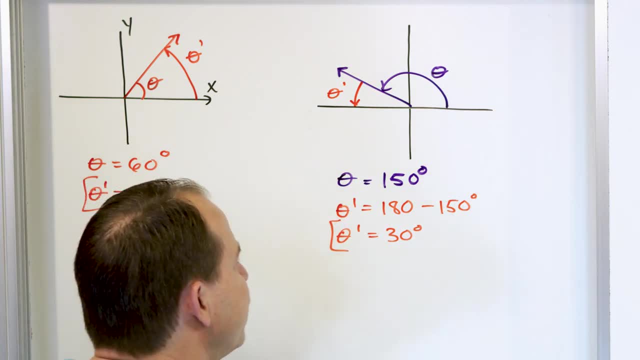 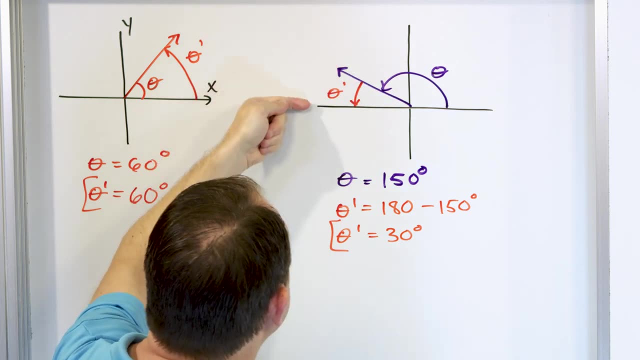 we're saying how many degrees is it from here to here? But we know that if this is 150 and this is 180, the difference between them must be 30 degrees. So what you're really going to do to find the reference angle? 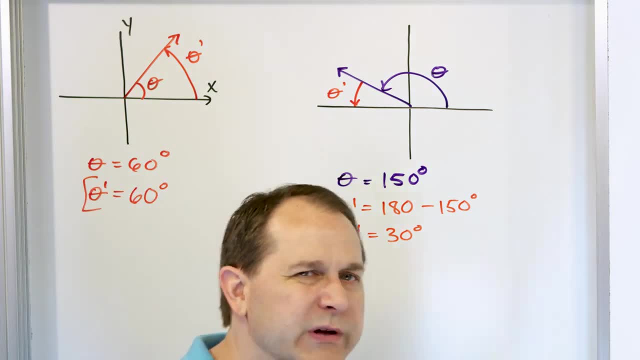 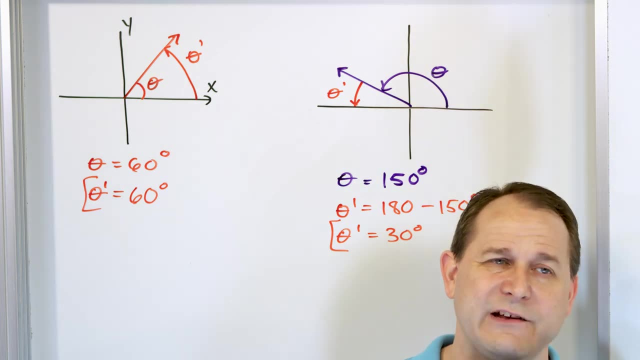 if it's obvious, you'll just kind of know what it is. But to do math to it is you're going to essentially have to add or subtract something to figure out what that angle is. And what you're going to do is you're. 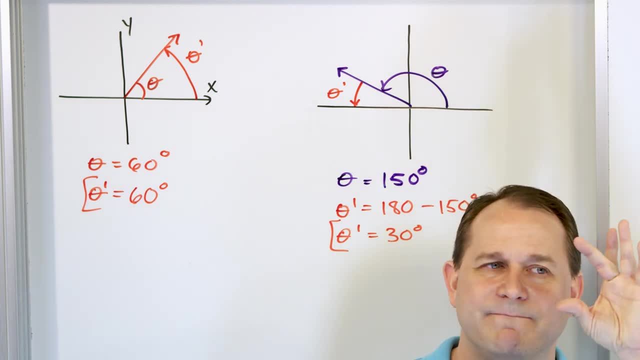 going to have to find the reference angle, And what you're going to do is you're going to have to find the reference angle, And what you're going to do is you're going to have to find what that angle is, no matter if it's on top, on bottom. 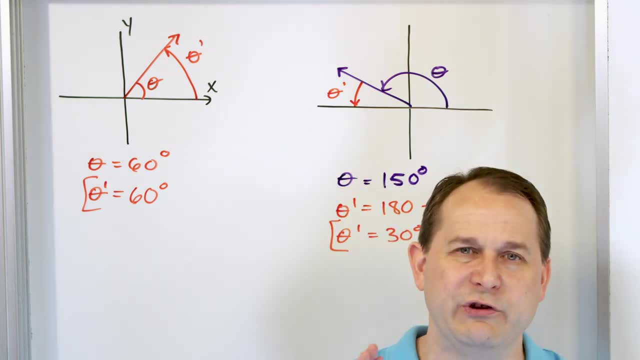 negative, positive. We don't care about any signs for the reference angle, We just want to know how many degrees if I took a protractor there to measure it would be. So let's do one in a different quadrant, Just to get some practice with something different. 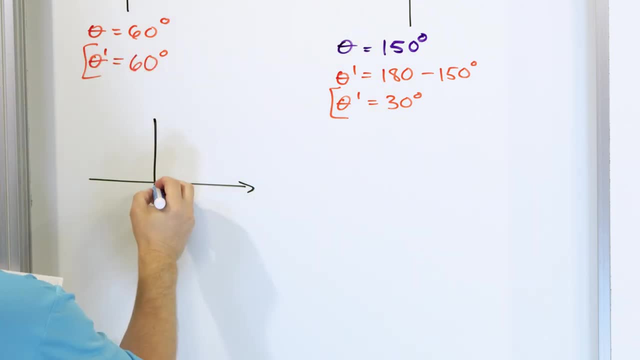 Let's say we have an angle over here in quadrant number 3.. Looks something like this, And that angle is measured from the positive x-axis, like it always is theta, like this, And I tell you that theta is 300.. degrees. And I'll ask you: what is theta prime? Well, theta prime is going to be the distance, or 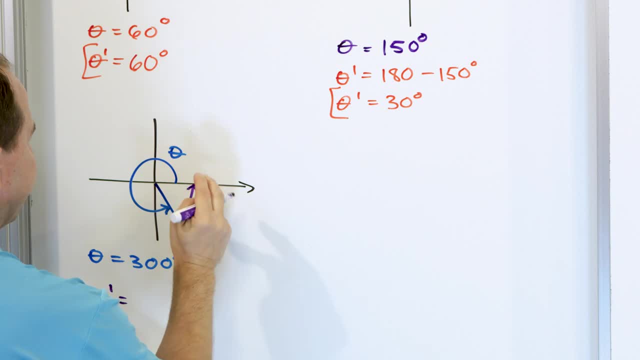 the angle from this terminal line to the nearest x-axis, which is this one. You're not going to measure it over here, That's farther away. It's always going to be an acute angle. So how do you figure it out? I mean, you know that if you go all the way around, this black line is 360 degrees. 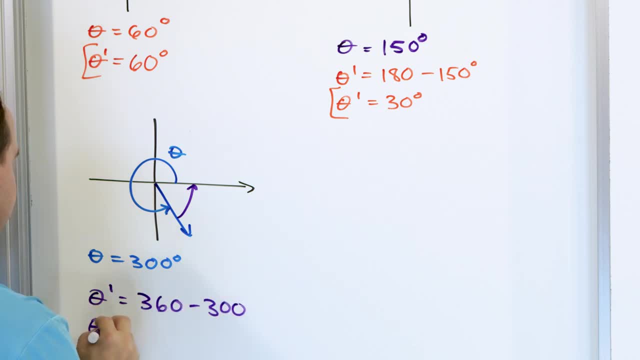 So then you take the 360 minus 300, and you'll get that theta prime is going to be equal to 60 degrees, And that's what it is. And you should do a sanity check just to make sure that this distance- if this is 270 here, the vertical line 300 is. here you get 60 more degrees to get to. 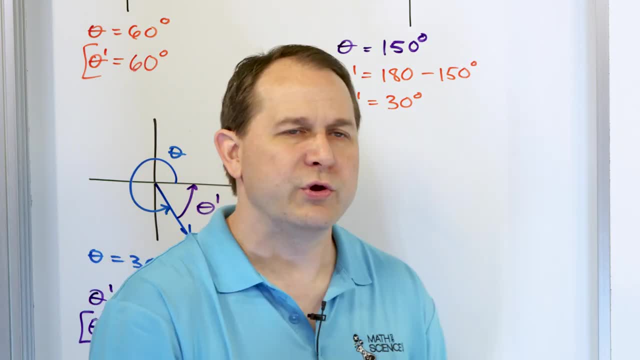 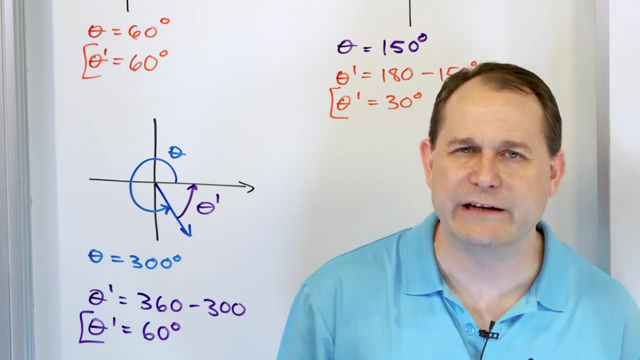 360.. It makes sense that that's what it is. So oftentimes when you're solving problems like this, especially later when we are doing the trig functions, the sines and the cosines, you're not really calculating the reference angle. You're not getting a calculator out. 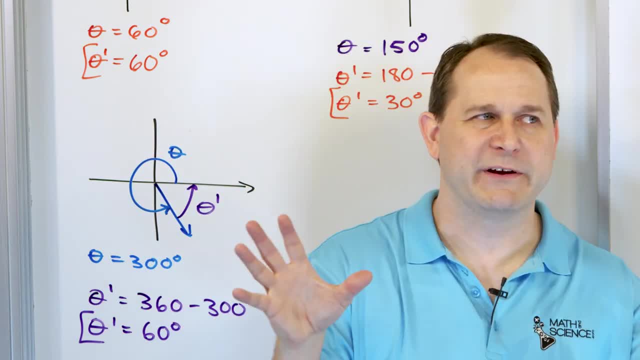 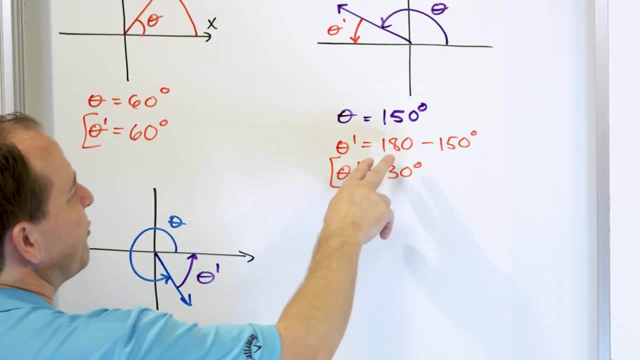 You just know where it is on the xy plane And you kind of know from experience how many degrees it is. You're just subtracting some number. Sometimes you're subtracting or adding 360.. Sometimes you're subtracting 180.. Basically, it just depends. Is it closer to this? 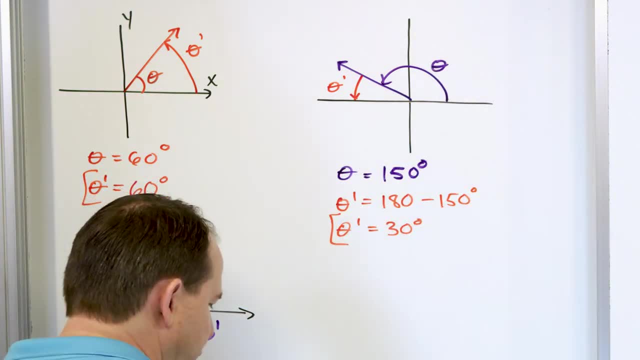 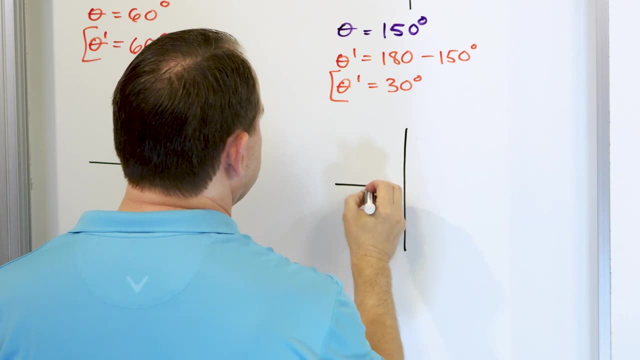 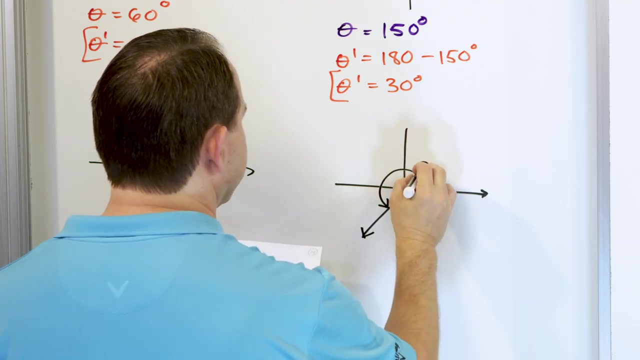 black line over here, Or is it closer to this black line That's going to determine what you add or subtract. All right, let's take a look at a different one. Let's say we have something over here in quadrant three like this: So the angle is theta here And we're saying that. 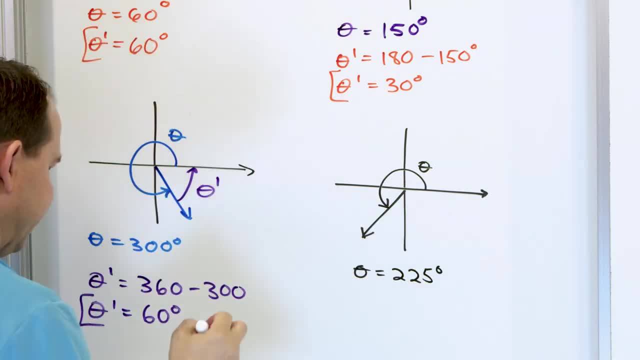 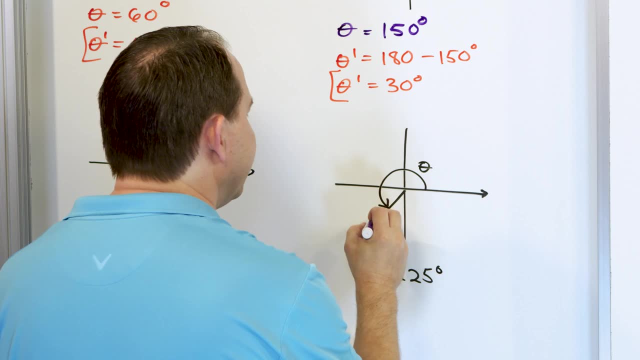 theta is 225 degrees. This is one of the ones we actually did over there. So if the theta angle is measured like this, how would you measure the reference angle? It's just the angle from this to the nearest x-axis. We label this theta prime. So what do you do? Well, if it says 225,. 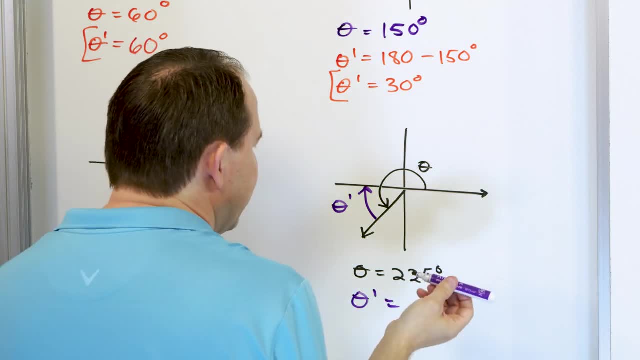 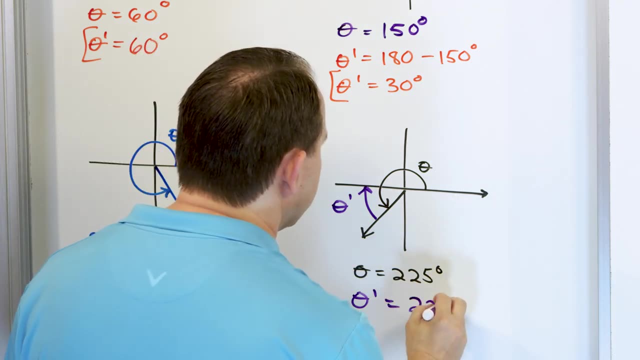 the nearest x-axis is this: We know this is 180.. So you either add or subtract 180.. But you're not going to add, That's going to get a really big number. You subtract 180.. So 225 minus 180.. 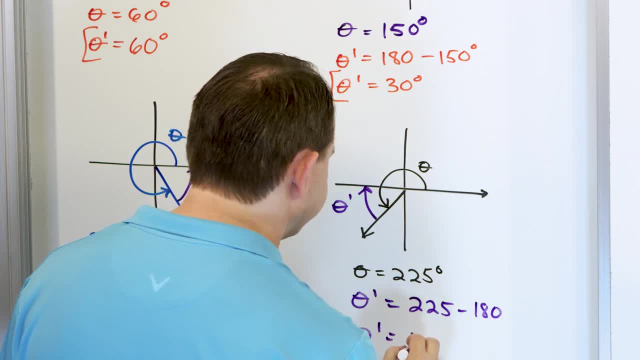 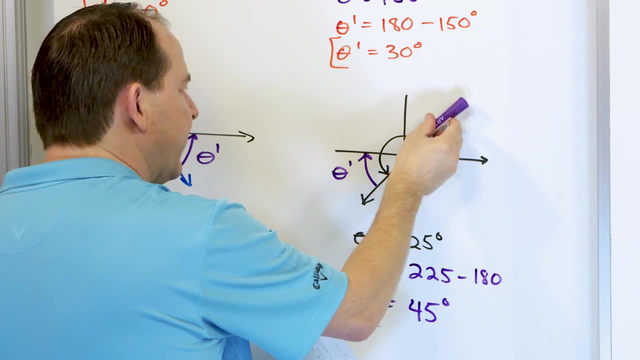 Theta prime, You're going to get 45 degrees And that's what it is And that makes sense, because you know that 225 is one of the. you know this is 45.. This is 135.. This is 225.. And you kind of. 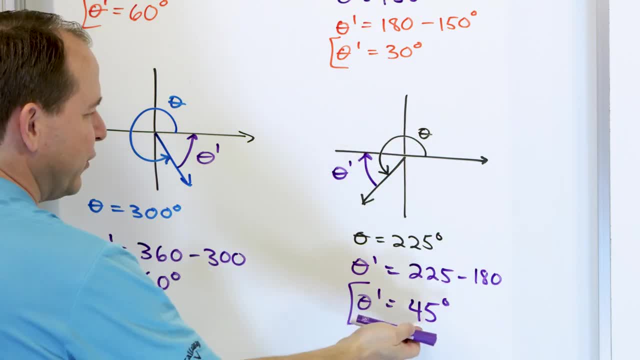 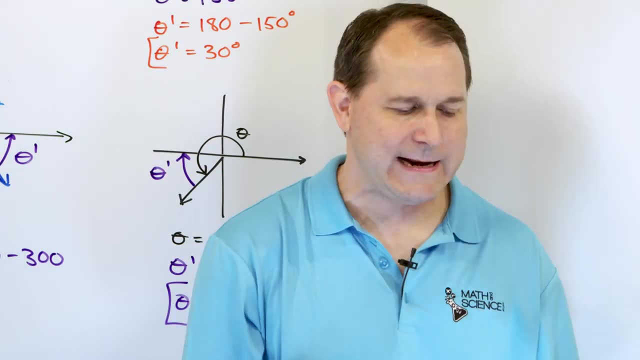 know those angles. So this one you know is at a 45-degree angle from the axis. So you kind of know it in the back of your mind, But you know showing math and subtracting and adding is a little trickier Now. these were reference angles when theta was positive, So you're going to get. 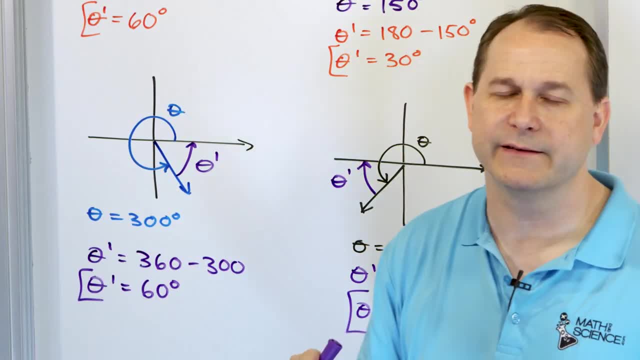 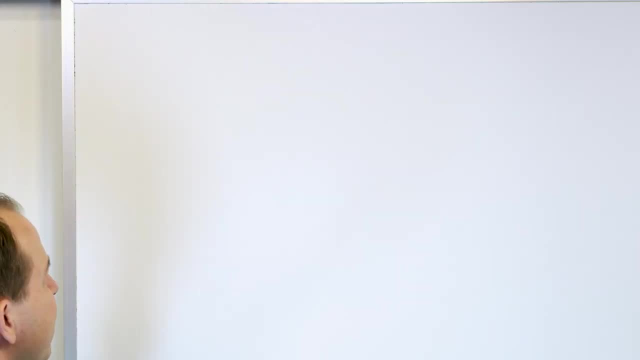 positive right. Theta was positive in all these cases, measured from the x-axis. What happens if the original angle is negative? Does it make it harder or not? Just remember what you're doing is no matter what you actually mathematically have to do. you just want to know what the angle is. 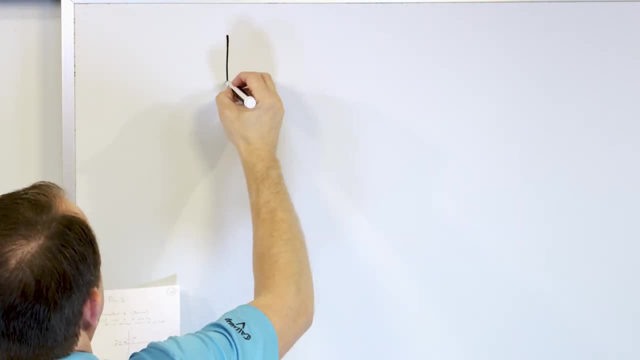 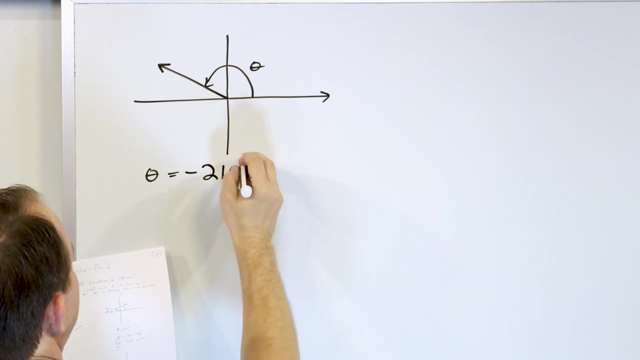 between wherever you're at in the x-axis. So let's say that we have something like this Over here, we have an angle like this And its measurement is: we call theta, And then theta is defined to be 210 degrees. So actually I made a mistake. Let me kind of subtract that I shouldn't have drawn. 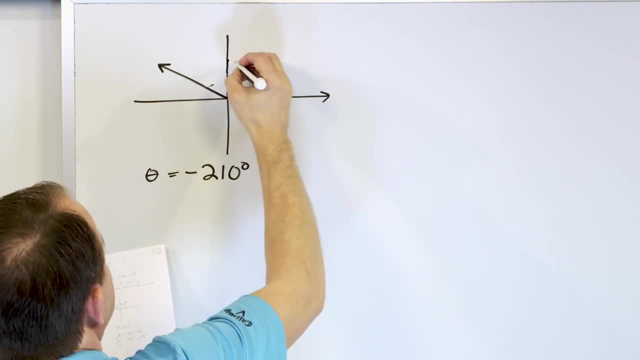 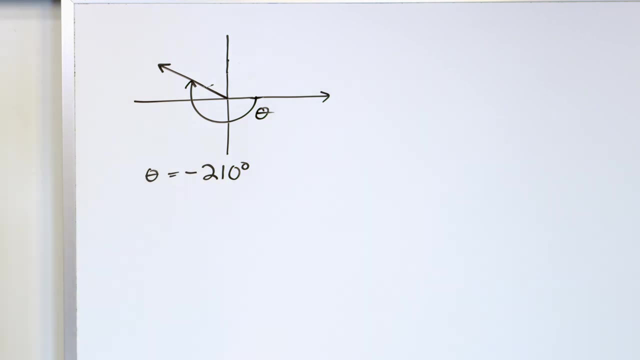 that in this problem. Sorry about that. What I'm really trying to say is the terminal side is there, but really it's measured here. Now this is called theta, And theta happens to be negative. So when you think about it, I mean it makes sense If you go this direction. 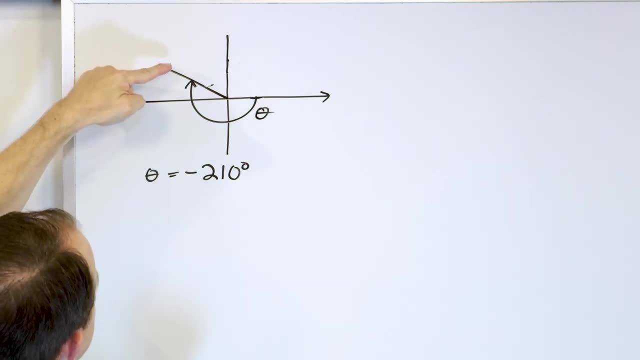 this is negative 180. So a little beyond negative 180 is up there. Now again, I think you probably already know the answer just by looking at it. But the terminal or the reference angle would be right here, theta prime. So what do you do? A lot of students don't know, Should I add or? 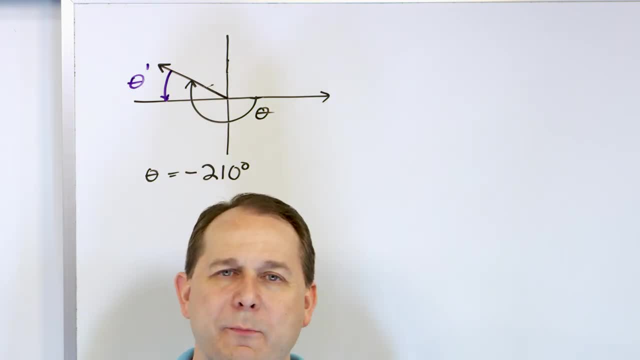 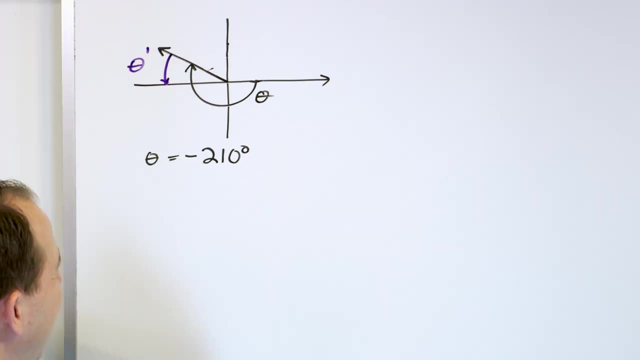 subtract. Well, ultimately, no matter if it's negative measure or positive measure, all you want to know is: how many degrees is this? So, yeah, there's a way to do it with negative numbers, But ultimately, what you need to do is say: well, OK, it's going to be this: 210 minus 180.. Those are. 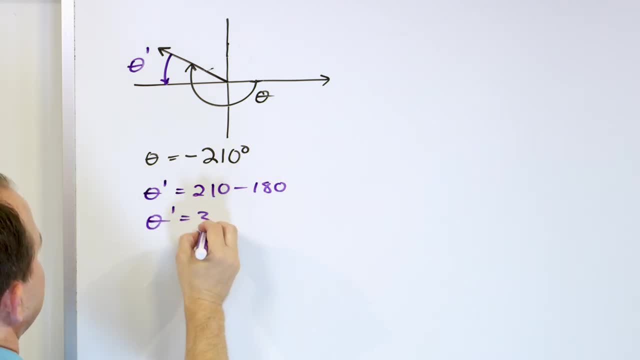 the two relevant numbers. If I subtract them, what I'm going to get is 30 degrees, which makes sense. if I go in the negative direction and land here, it's negative 180. But I go another 30 degrees up to get to negative 210.. So it is a 30 degree angle And you can convince yourself of that. 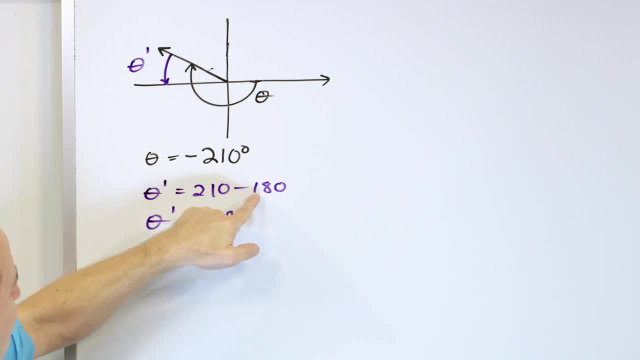 But still, sometimes people aren't sure why. Why did I take the negative away here? Why did I do this? Well, the answer is: the angle measure is negative 210. And then the line over here is negative 180. So you could subtract them: Negative 210 minus a negative 80, which would be plus 80.. 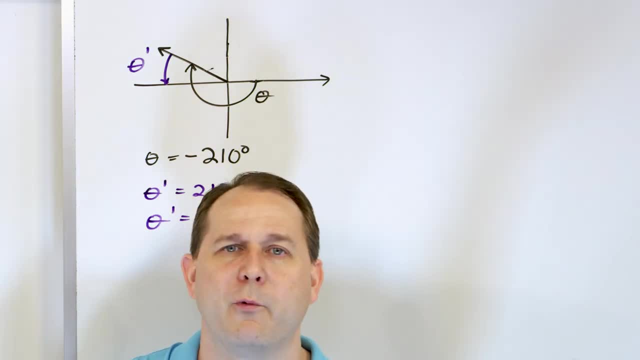 And you would get negative 30 degrees As the angle. But we strip away all signs. We don't care if I'm measuring going up or coming down. The negative sign tells me which way I'm measuring- going up or coming down- But I don't. 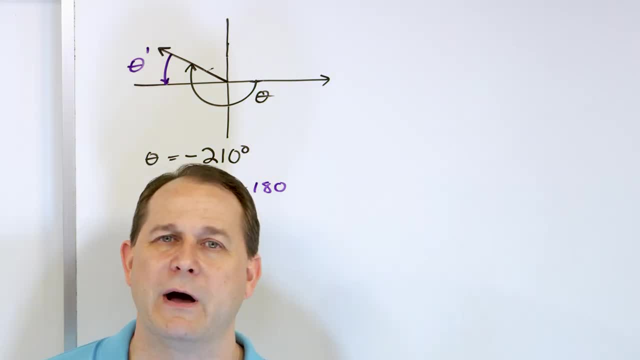 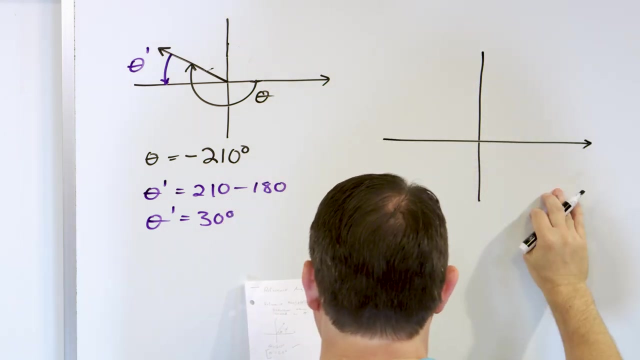 care about that, I just want to know what the angle is. is a positive number, So you would strip away the sign anyway. I find it much easier just to take the numbers and subtract them, get a number out of it, All right. next problem: What if we have something like this, And we have 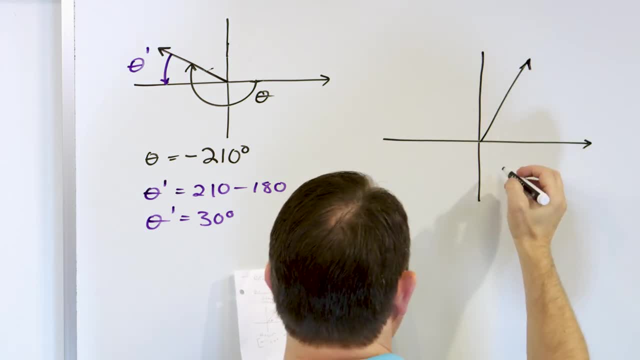 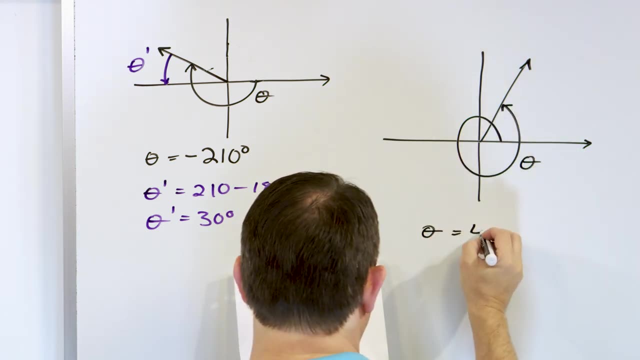 something over here Looks like it's in quadrant one And the angle here is not going to be negative, but it goes around all the way around like this: This is theta, And we say that theta is equal to 420 degrees. What is the reference angle? 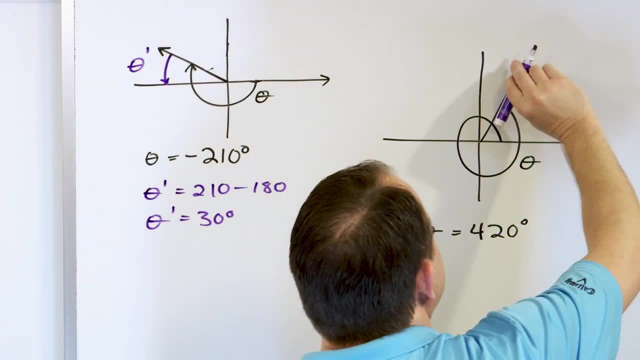 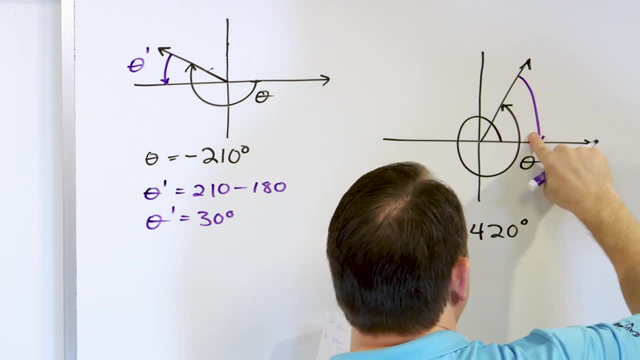 First of all, on the diagram, what is the reference angle? It's the smallest angle to the nearest x-axis, So something like this: This is the angle that I want, right here. You could draw the arrow down here. You could draw the arrow up here, It doesn't really matter. 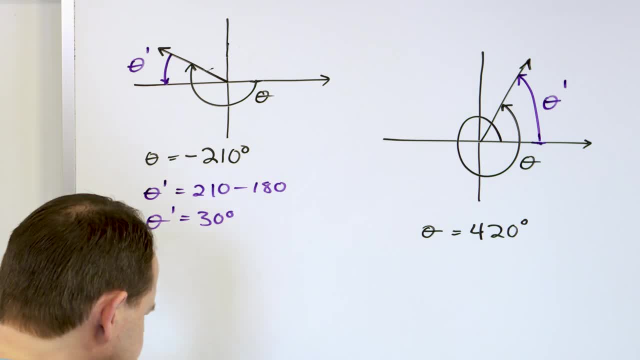 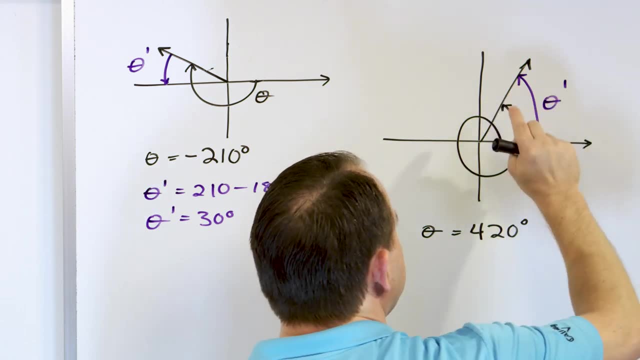 too much, But anyway, this is theta prime. That's what I'm after Now. it's a big angle. It goes all the way around 360.. Then it goes some distance up. I want to know what this extra distance is up. That's going to be theta prime, All right, So, since it goes all the way around, 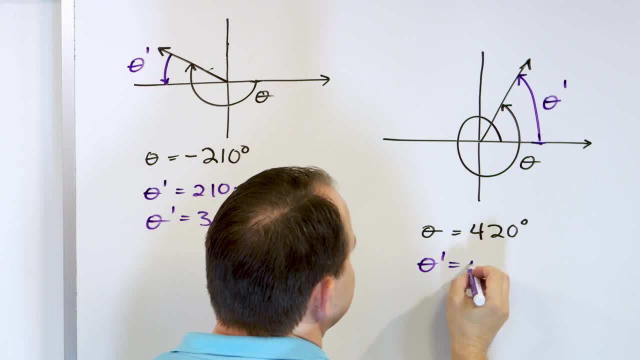 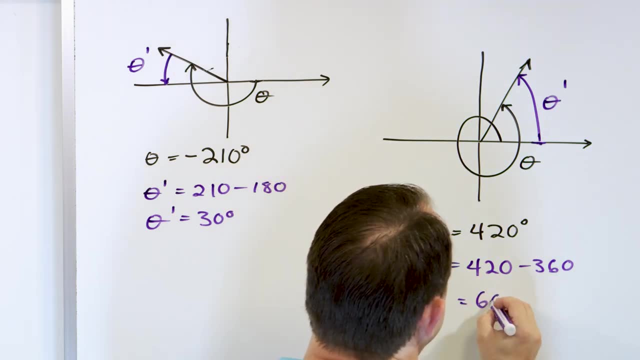 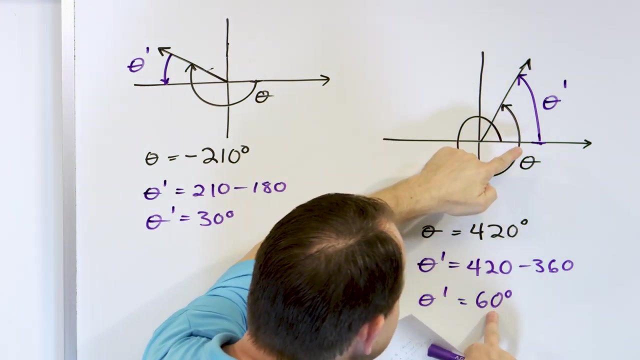 and you're measuring to the black line. what you do is you say theta prime is 420 minus 360.. Theta prime is going to be- there's going to be 60 degrees. And then you look and see: does it make sense If I go all the way around to 360, 360 plus 60 more is going to be going up to. 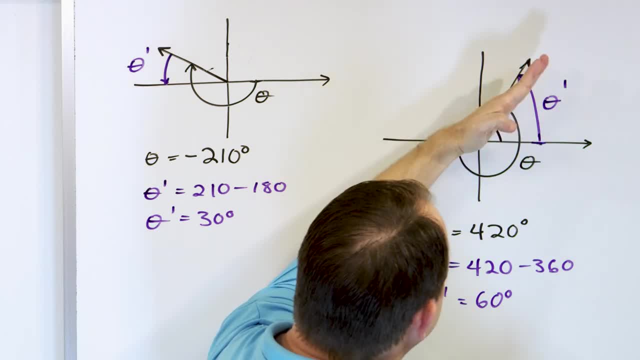 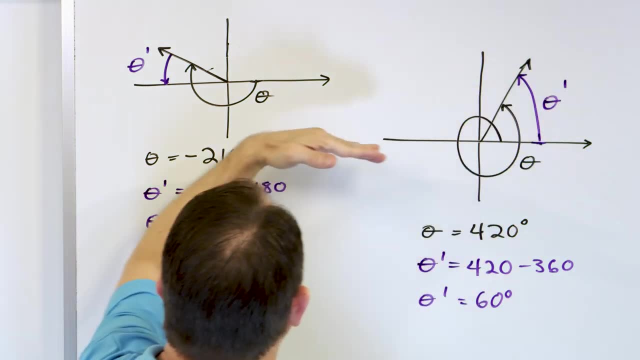 420, which is where it is. So all I'm after is: what is this angle measure here? So sometimes you subtract 360.. Sometimes you subtract 180. It just depends on if the terminal side is over here somewhere. or if the terminal side is over here somewhere, Strip away all signs. strip away. 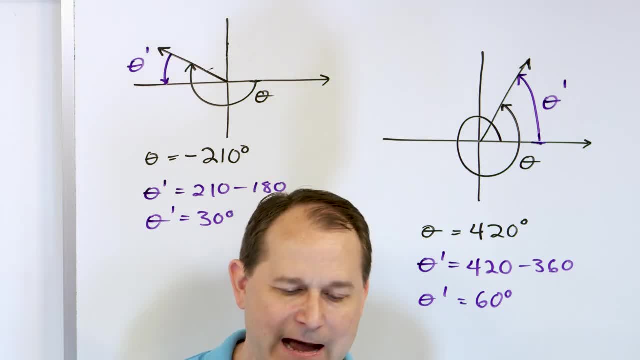 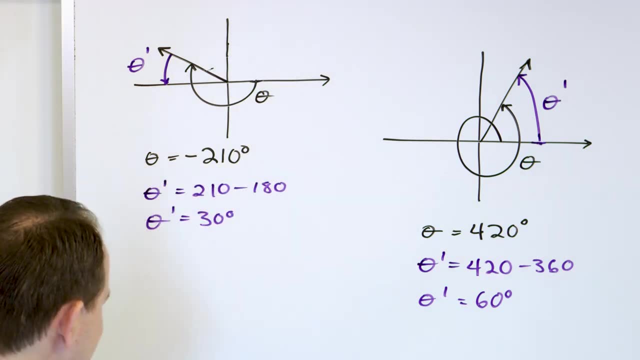 negative numbers and all of that, and you're going to get the reference angle. Now we get to the important part: Why are we calculating a reference angle? Why do we care? Here's the reason why. Let me do a little bit of a lecture and then we're going to solve a couple of quick. 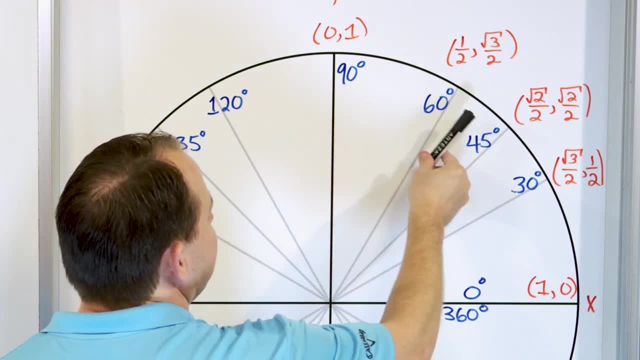 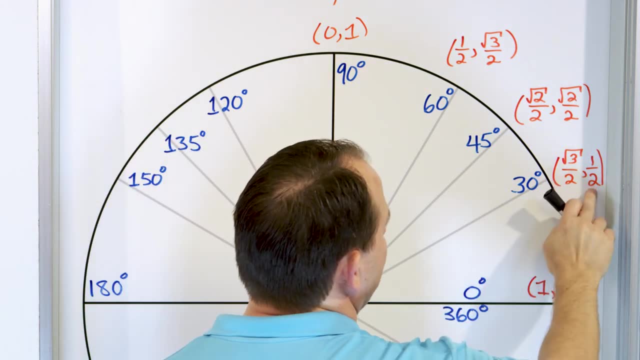 things In the past. we have learned how to find the sine and the cosine of these numbers over here, these angles right, So let's pick one that we know really well. Sine of 30 is one half this number right here. This is the x, the cosine value, and this is the sine value. So we know that. 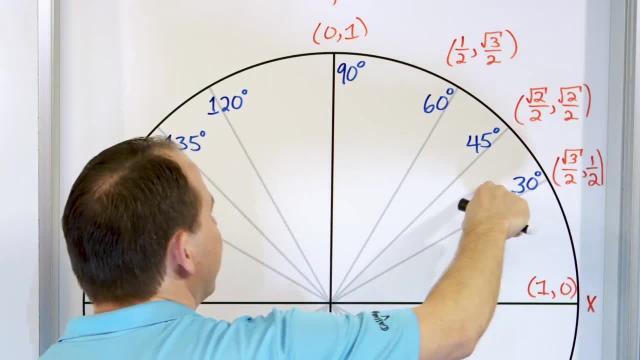 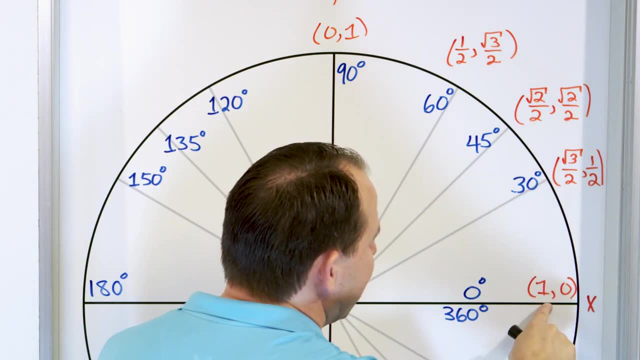 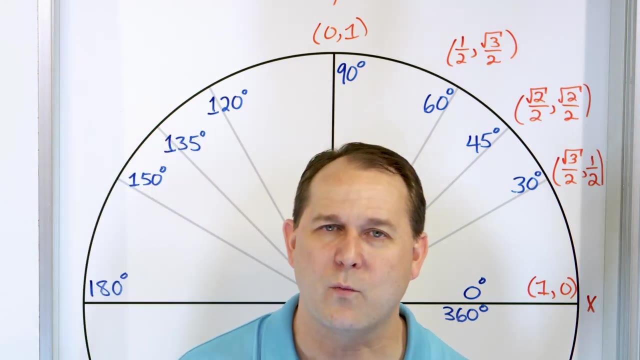 sine of 30 is one half. That means that the projection over here is one half right. And we also know that the cosine of this number is the square root of three over two. That's the value of the x-axis. So we know a long time ago that the sine is the projection onto the y-axis. Sine goes. 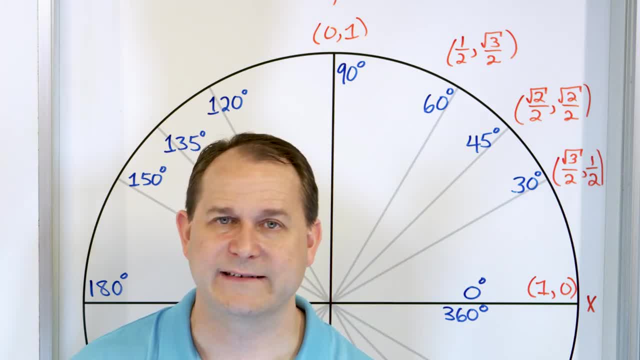 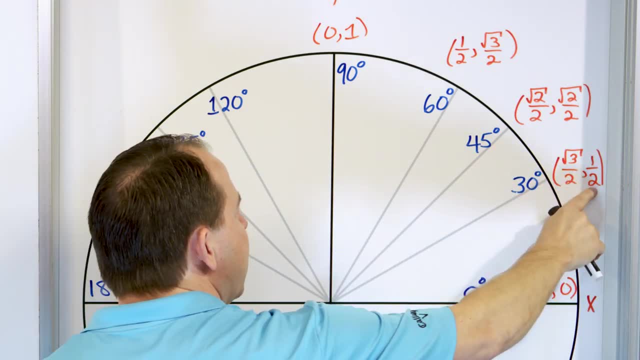 with y And the cosine is the projection onto the x-axis. It's just as if I shine a light on this hypotenuse and it casts a shadow, This much is going to be one half. And if I shine a light down and it cuts and makes a shadow here, this distance, since it's a unit circle with a radius. 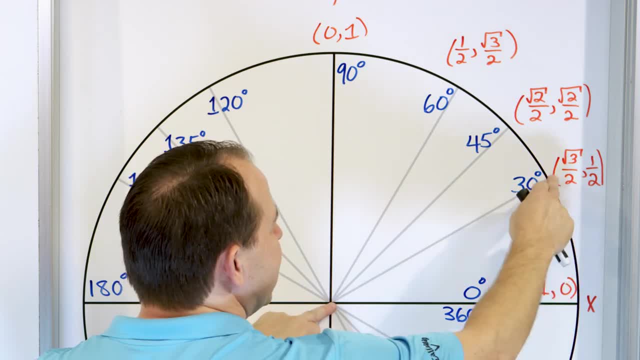 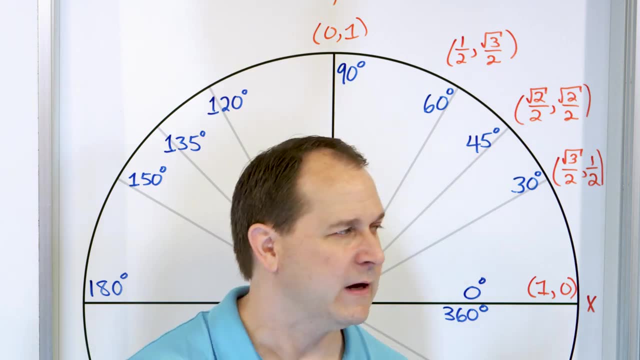 of one will be square root of three over two. It's about 0.866 or so, And so this is the shadow that would cast right there In quadrant one. all of the projections are positive because the x-axis is positive and the y-axis is positive. 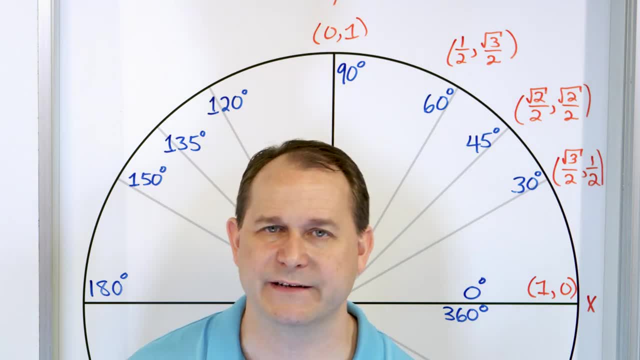 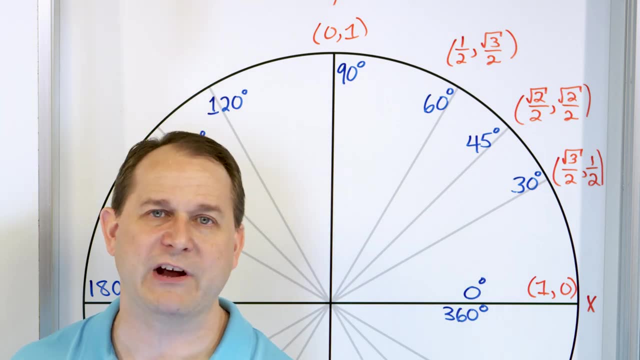 But in the other quadrants, x and y- are not positive. So in the other quadrants the sine can give you a projection that's negative and the cosine can also give you a projection as negative. Let me show you what I mean. We all know that this is 150 degrees, We know that right. So if I say 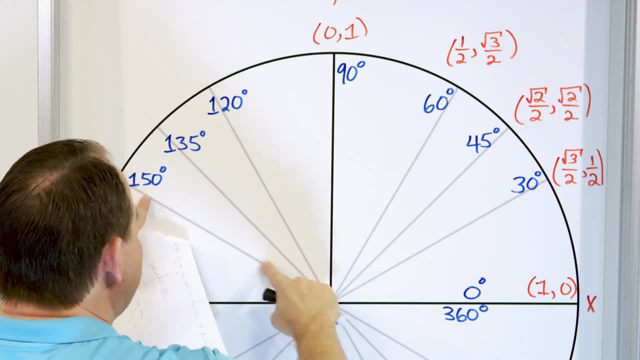 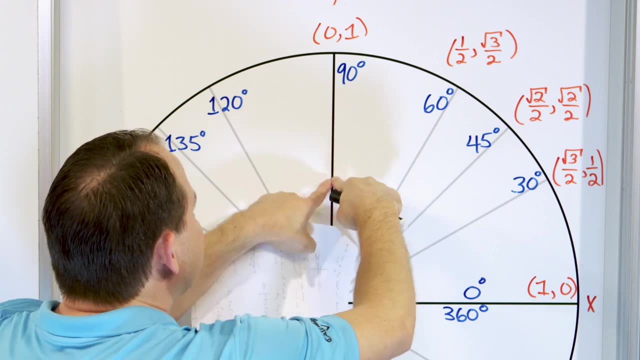 what is the sine of 150 degrees, Since it looks exactly like the mirror image of this one. you know that if I shine a projection like this and it casts a shadow right here, it's going to be the exact same value. if I cast it from here onto the 30 degree because of 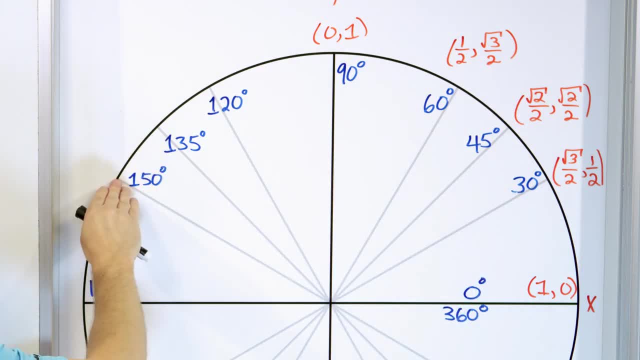 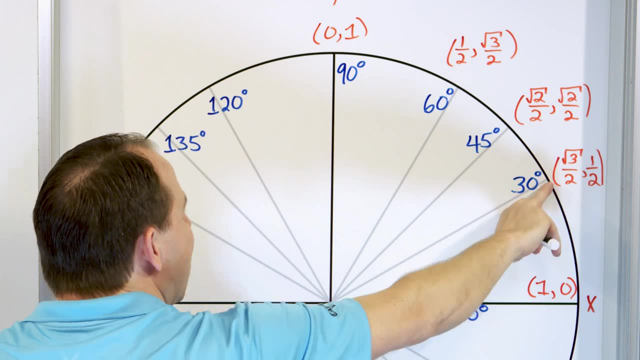 symmetry, So it's going to be one half. So we now know that the sine of this 150 is going to go land on the same place, the positive y-axis over here. It's going to give me the same sine, The sine of. 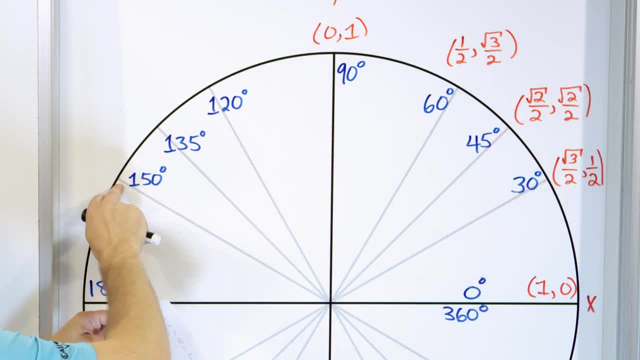 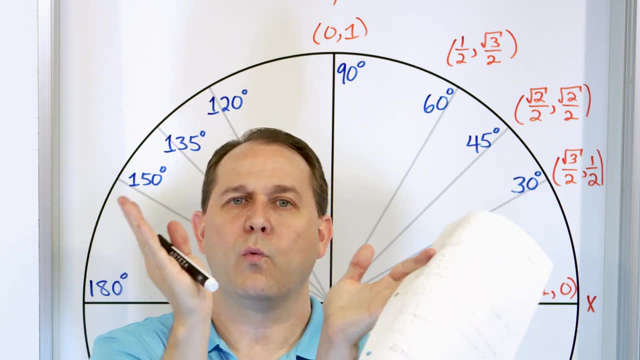 is the same exact thing as the sine of 150, because the projection on the y-axis is exactly the same for both of those angles. So if you're looking at angles in quadrant one and two, the sines of those angles are always the same. 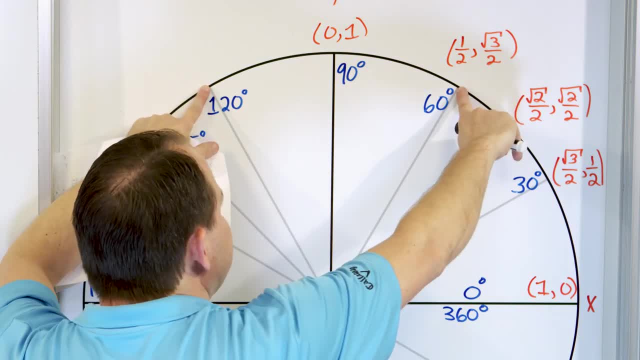 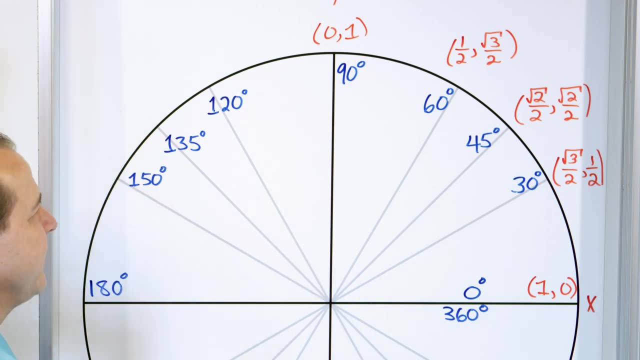 The sine of 120 is exactly the same as the sine of 60, because if I take a projection over here and I take a projection over here, the sine, which is the projection on y, is exactly the same for those. But let's go and examine this one and this one again. The cosine over here was the projection. 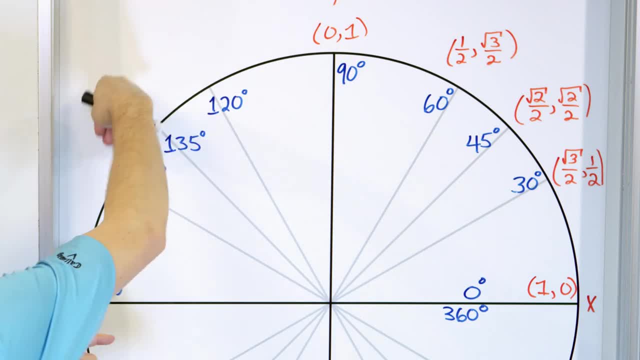 over here. That's positive values of x. But the projection down here on the x-axis is not positive. These are all negative values of x. So if I shine the value down it's going to cut over here. I expect to get a negative cosine. 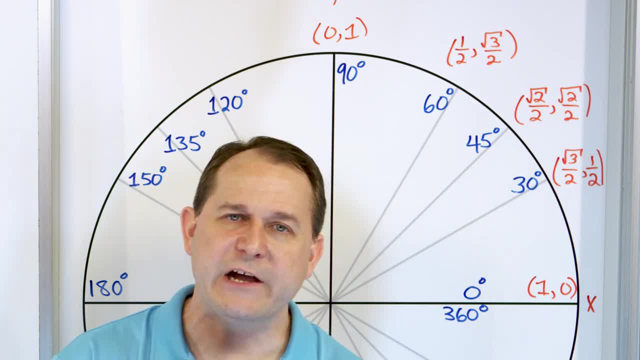 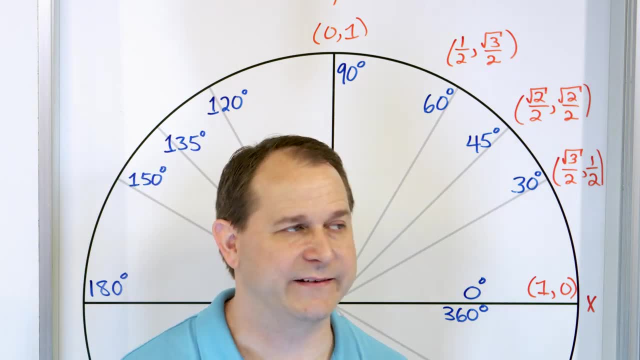 That is the secret sauce of sine and cosine. To figure out what the sine of a value is, you figure out where it is in unit circle and you project it and see where it lands on the y-axis. If the projection is anywhere up here, the sine is a positive number somewhere between zero and one. 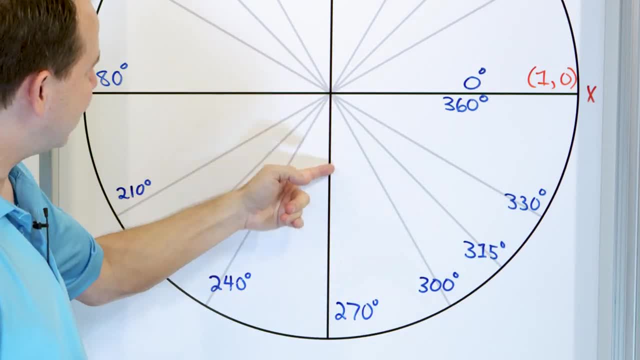 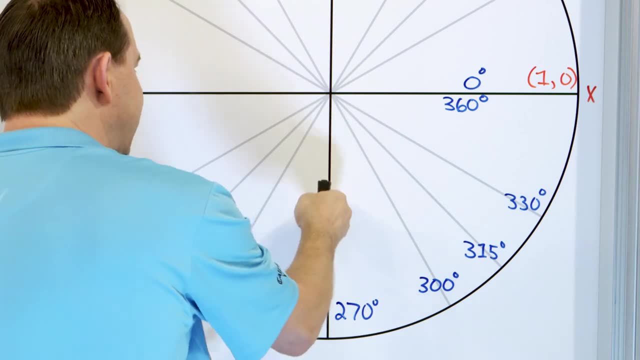 If you are down here and you do a projection on the y-axis, then the y-axis is negative and you're going to get a negative cosine. You'll always get negative signs for all of these angles because all of their projections will all be a negative y. 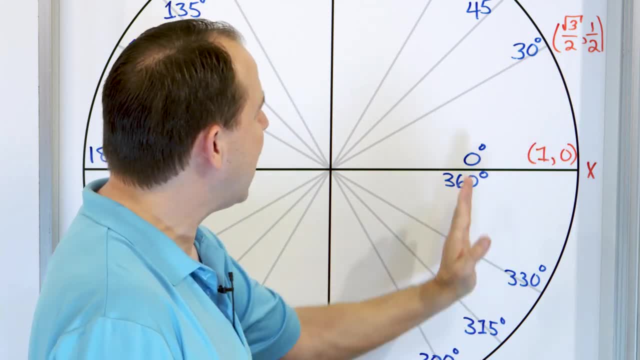 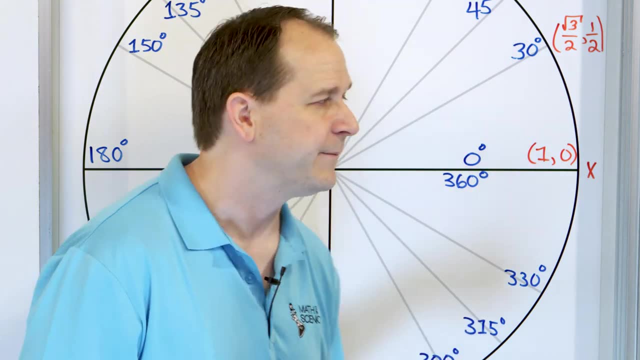 Likewise anybody over on the right hand side, the positive x-axis. any of these angles will give me projections that are positive, which means the cosines will be positive, And over here the cosines will always be negative for all of these angles, all the way over here, because any 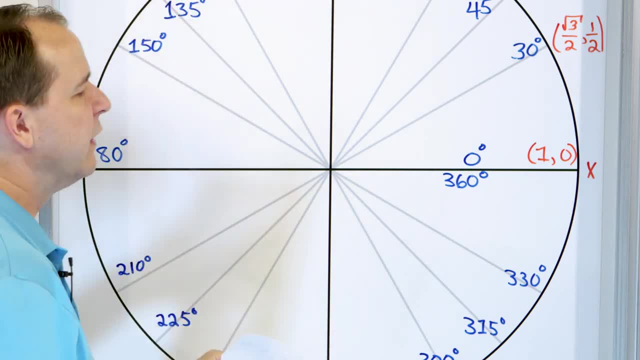 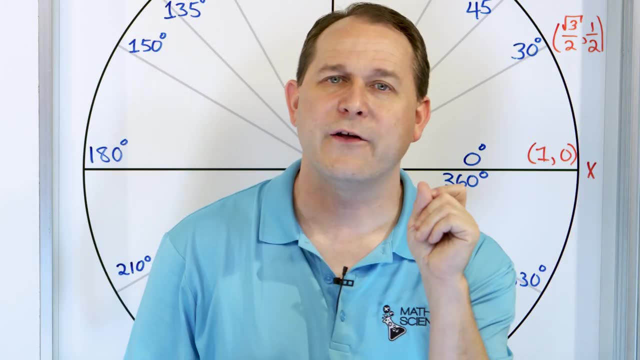 projection from down below or up above is going to land over here. So the secret sauce of figuring out what the sine or the cosine is of any of these angles around the unit circle is to figure out the reference angle first, Because if I know, the reference angle here is 30 degrees. 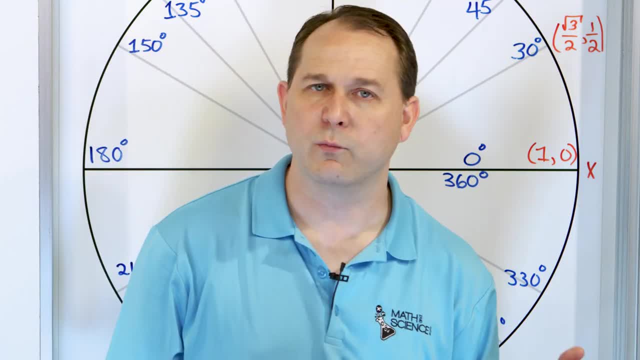 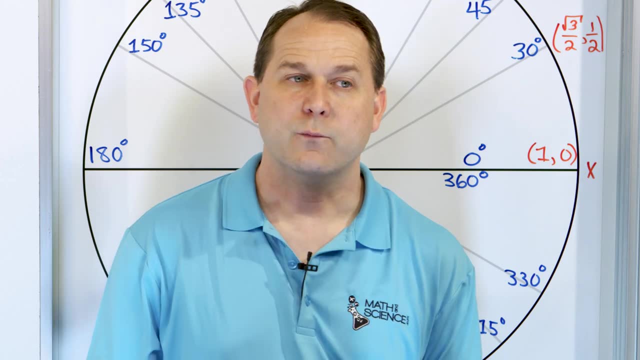 and I already know what the sine and cosine of 30 degrees is from quadrant one, then I know what the number of the sine and the cosine is. The numbers are all written in red around here around the unit circle One half. you know the sine is one half of 30 degrees and the 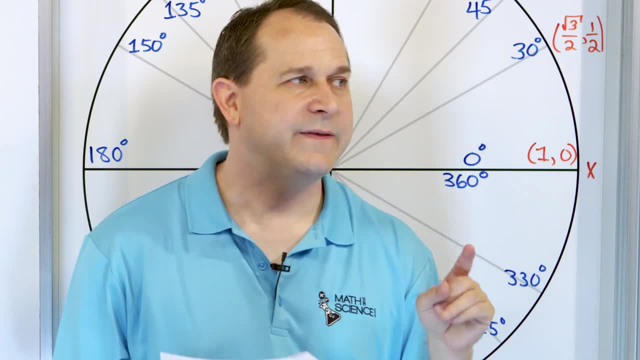 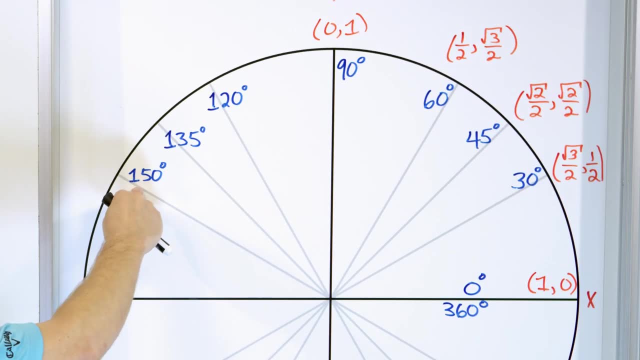 cosine is square root of three over two. But in the other quadrants the sine and cosine will have the same numbers but different signs. So we could for instance say: what is the cosine of 150?? Well, the cosine of 150 is the projection down here. We know the cosine of 30 is square root of three over. 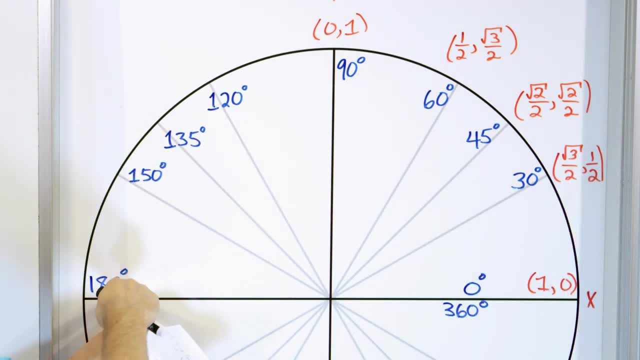 two. So we know the cosine of 150 must be the same number Because of symmetry it's square root of three over two. but this projects down here to negative square root of three over two. So the cosine of 150 is negative square root of three over two. The cosine of 30 is positive square. 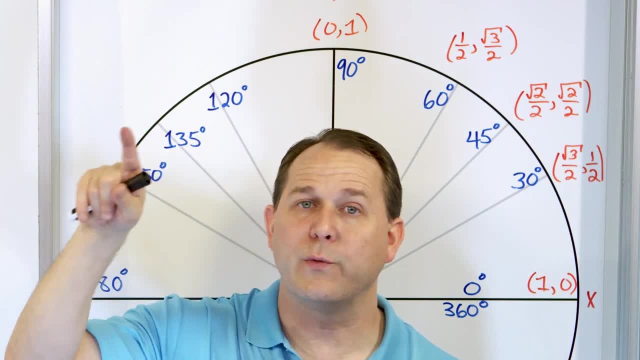 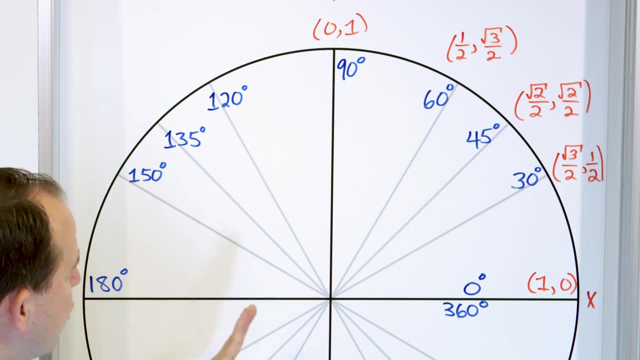 root of three over two. And so that is basically what we're going to do. We're going to walk around circle And we're going to figure out the sine and the cosine, first by figuring out what is the reference angle. What is the reference angle? Once we know the reference angle, we know what the sine. 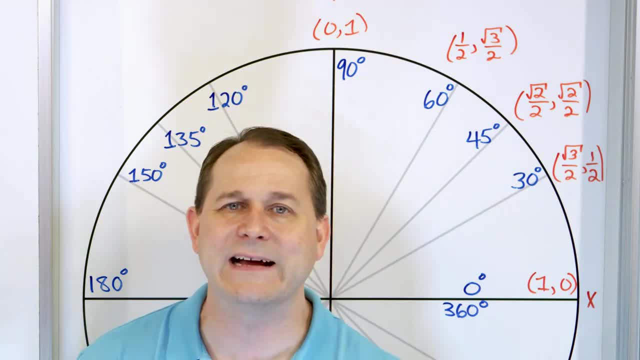 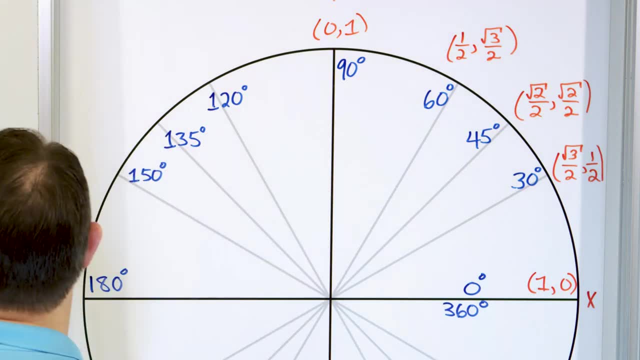 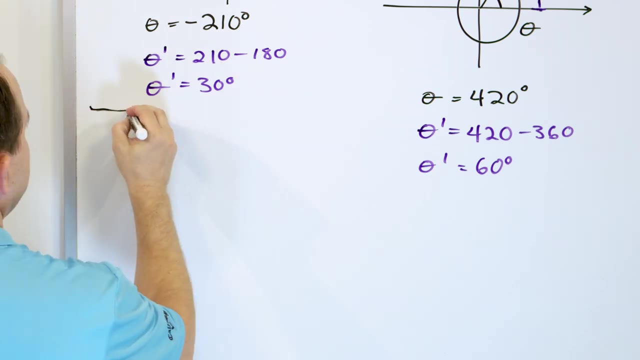 and cosine numbers are in quadrant one, but then we'll just take those numbers and we'll put signs on them, either negative or positive signs, to figure out what actually is going on. So, with that understanding, let's go and try to make some sense of the next problem. This is a great set of 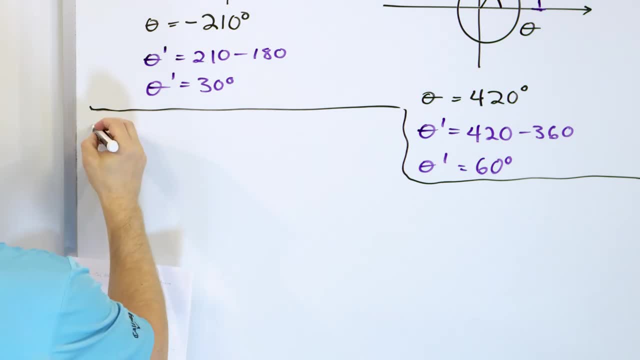 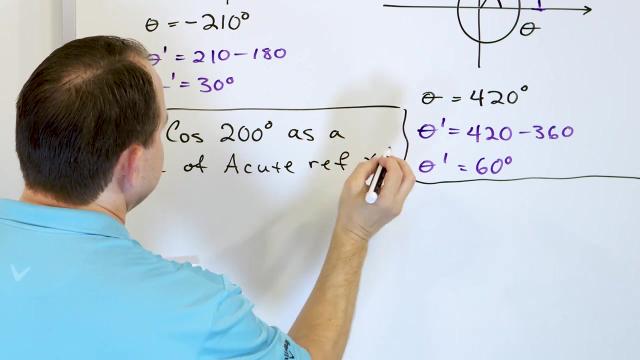 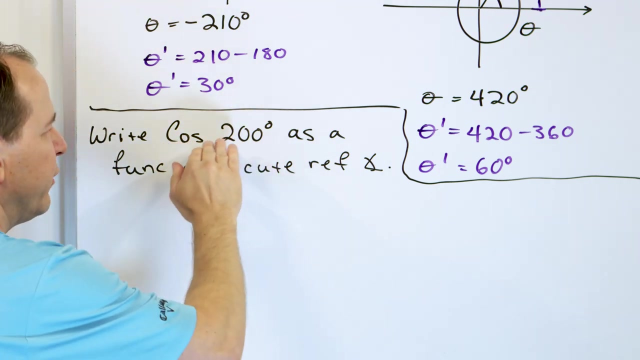 problems coming up. They're extremely important. okay, So I want to write cosine of 200 degrees as a function of some acute reference angle. Now this problem looks really hard, but actually we know everything needed to do this. We want to find write the cosine of 200.. Notice that 200. 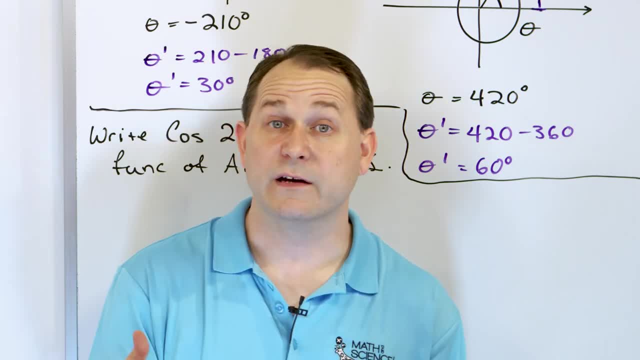 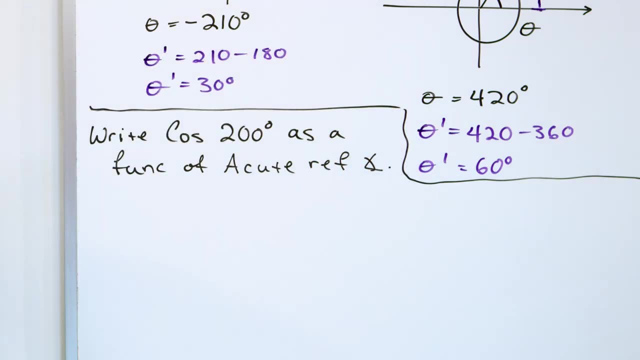 is not an angle that we know so well in the unit circle. But still, once we know the cosine of 200, how do we write it in terms of a cosine of some other reference angle? The very first thing you need to do is draw a graph and figure out where on the unit circle 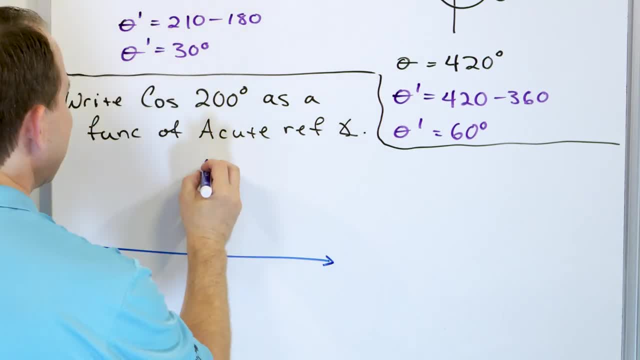 this 200 is so that you can visualize it. I'm telling you right now, in the beginning, if you're not drawing pictures, you're going to get something wrong. So you know that this is 0,, this is 90, this is 180, this is 270.. So 180 is here. So a little bit beyond that is 200 degrees. 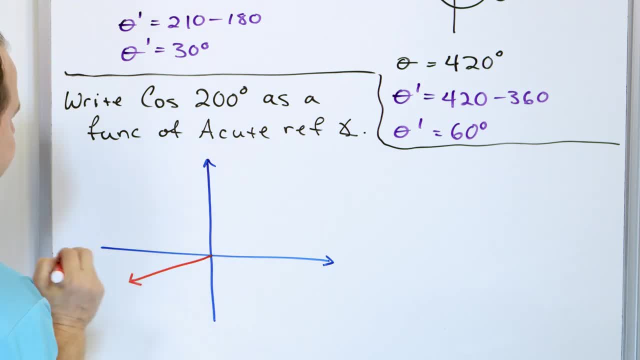 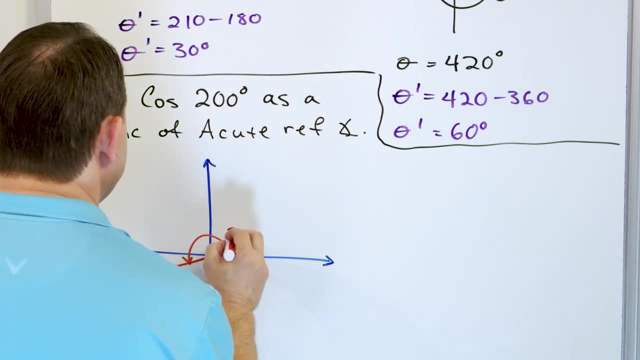 So let's draw our terminal angle over here like this: So we know that this angle is 200 degrees. So let's draw our terminal angle over here like this: So we know that this is 180, right, And we know that this angle right here is measured as 200 degrees, And because it's 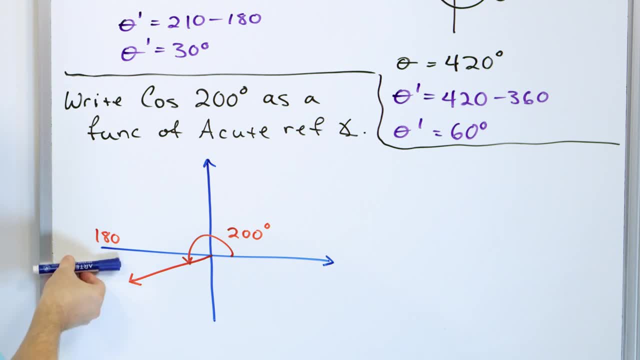 200 degrees, we know something really critical: What is the reference angle? here We just studied what the reference angle is. It's the angle to the positive x-axis, This or not the positive x-axis, the nearest x-axis, This angle, right here we call it theta prime, the reference angle. 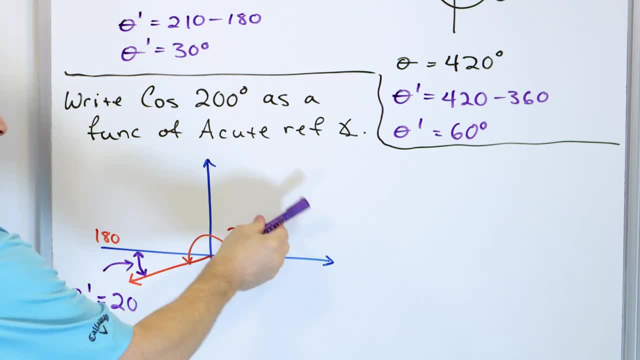 is actually 20 degrees. How do I know that? Because this thing is 200 degrees and the nearest x-axis here is 180.. So we subtract and we get 20.. If you get a protractor, you're only going to measure a. 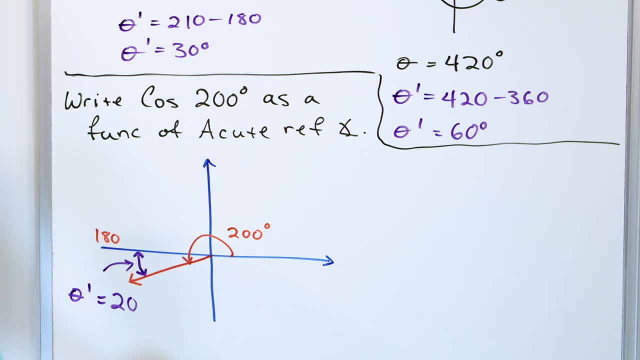 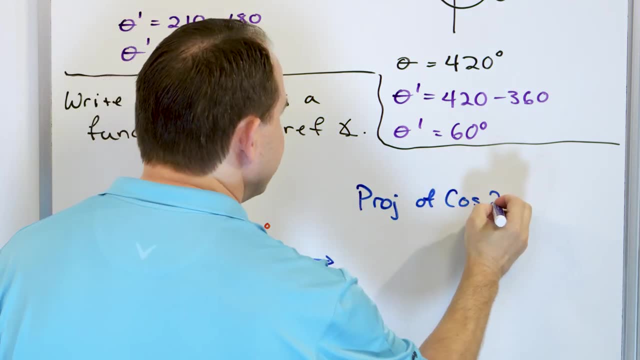 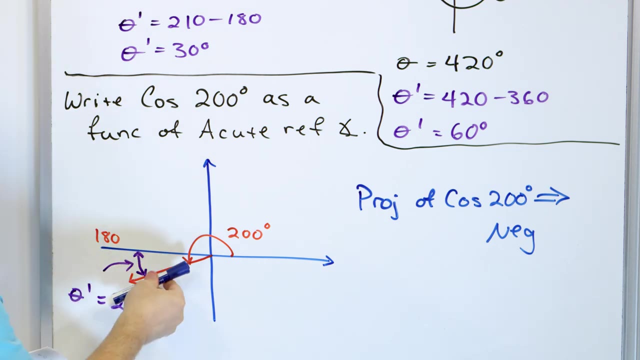 20 degree angle. Now here's the critical piece of information: The projection of cosine 200 degrees is going to be negative. Remember, cosine projects to the x-axis. If this is the angle, if we shine a light and project it to the nearest x-axis, the x values are all negative over here. 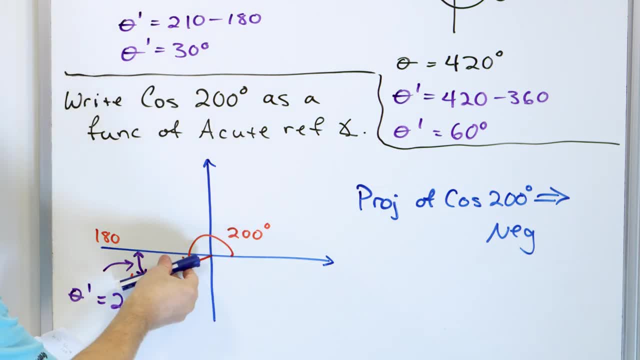 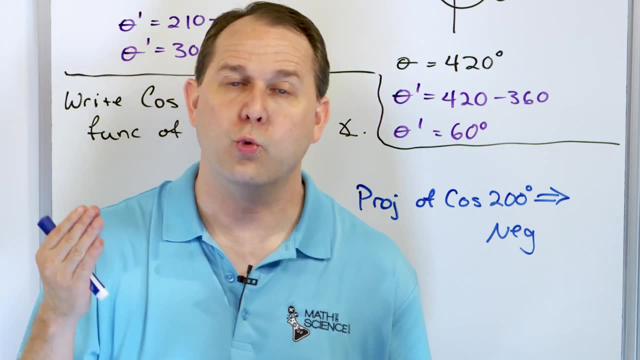 The x values are positive over here. but the x values are negative over here. So this projection is going to project onto the negative x-axis. That means the cosine of that angle will be negative. All you do is you look at where it's at, you project it on the x-axis for a cosine question. 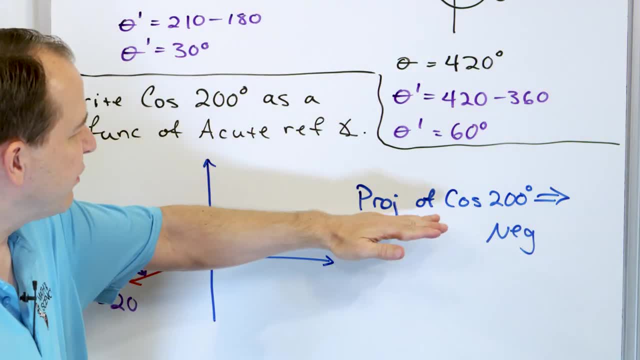 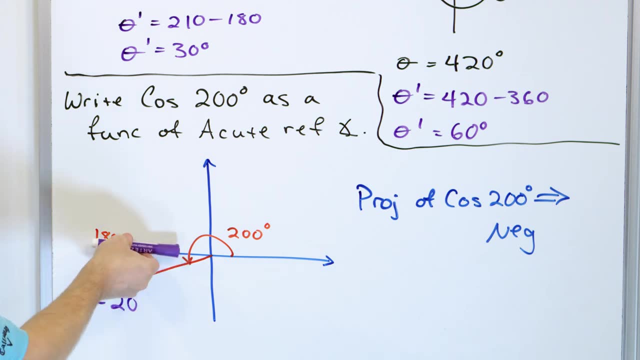 and if it's in the negative x-axis it's going to be a negative cosine. So the projection of this angle when you're taking the cosine is going to be in the negative axis there because it's projecting up to this guy right here. 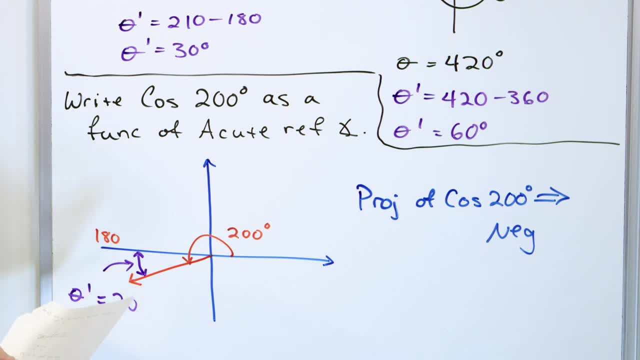 All right then. So the question then is what I want to do is write cosine of 200 degrees as a function of the acute reference angle. We now know the reference angle is 20 degrees, So what we're basically saying is that cosine of 200 degrees is exactly the same as negative cosine. 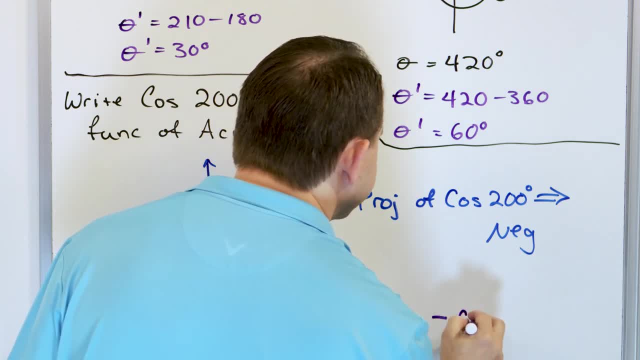 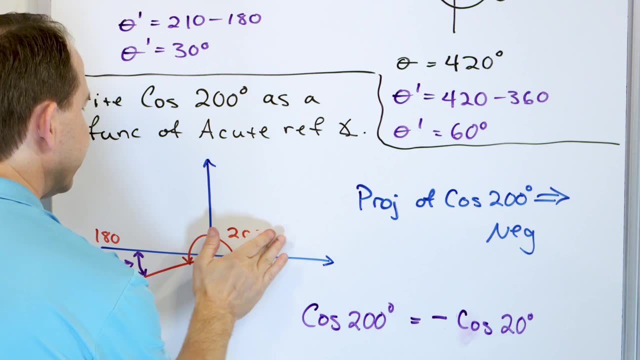 Whoops, I messed up already. Sorry about that Negative cosine of 20 degrees. Now let's break this down. Let's break that down for a second and make sure you understand. Let me actually get this out of the way because I'm going to need to draw something up here. 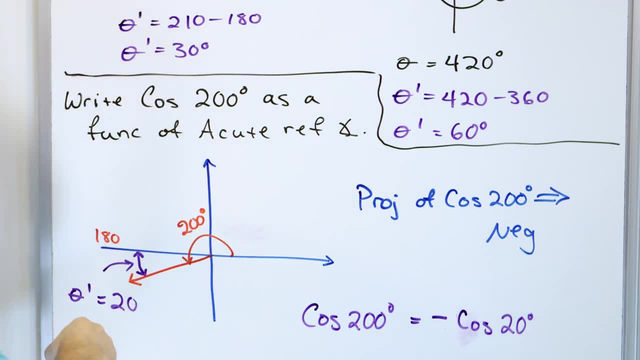 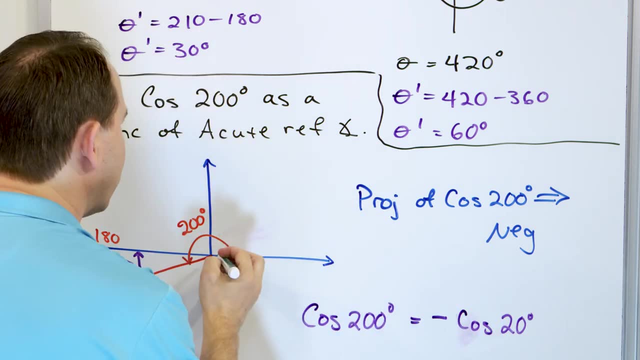 This is still a 200-degree angle. right. It's negative of cosine of 20.. Why? Because what does a 20-degree angle look like? A 20-degree angle- if I were to draw it in quadrant 1, is going to look like this: 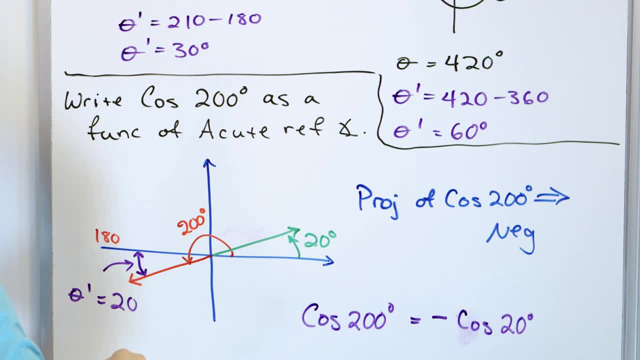 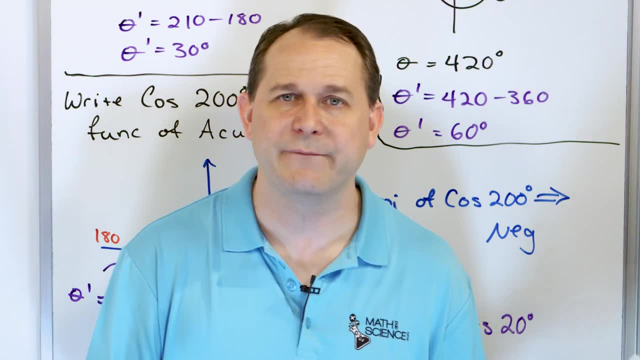 This angle is a 20-degree angle in quadrant 1.. So if I take like, I know that I don't know in my mind what cosine of 20 is, It's not one of the special angles, but I know that it has some value. 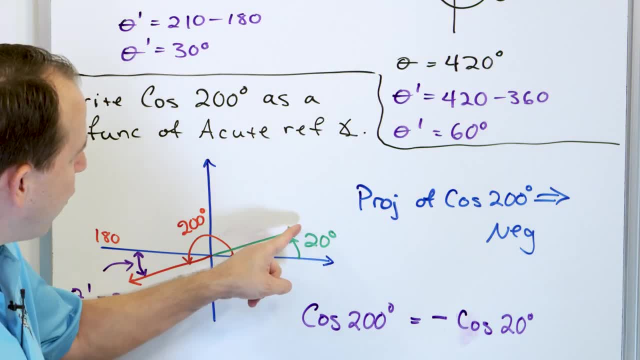 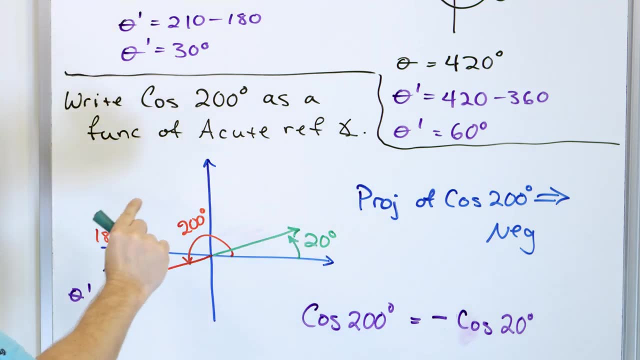 Right, I know that I can project it onto the x-axis. If I go figure out what this projection is, it's going to in the first quadrant. it'll give me some number And whatever that number is will be the exact same absolute value as the projection over here. 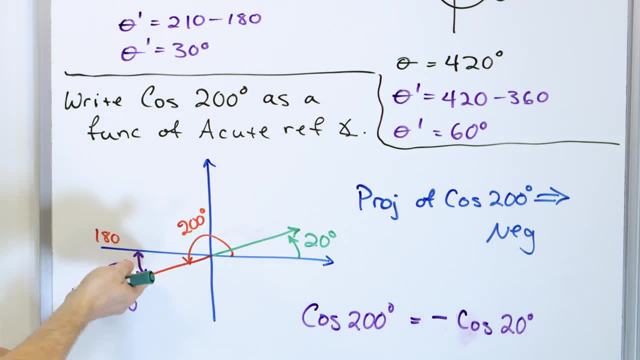 Because the reference angle, the 20-degree reference angle that's over here, the projection on this negative x-axis is going to be the same number as the projection over here. It's just: this one will be negative and this one will be positive. 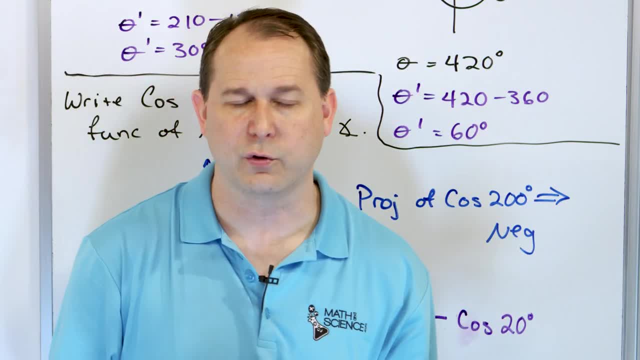 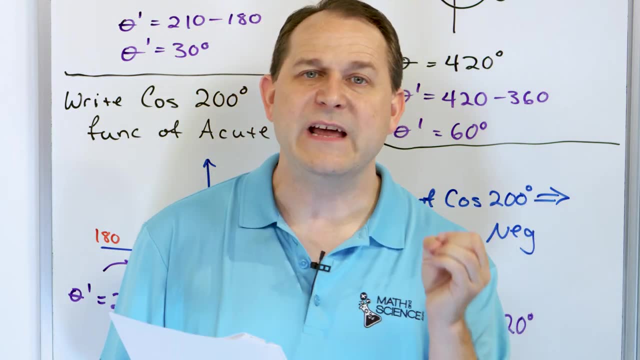 So what you do when you have angles on the other side of the unit circle is you figure out. you figure out the reference angle first, Then you take either the sine or the cosine of it and you get the value. Then you slap a sine on it, dependent on what quadrant it's in. 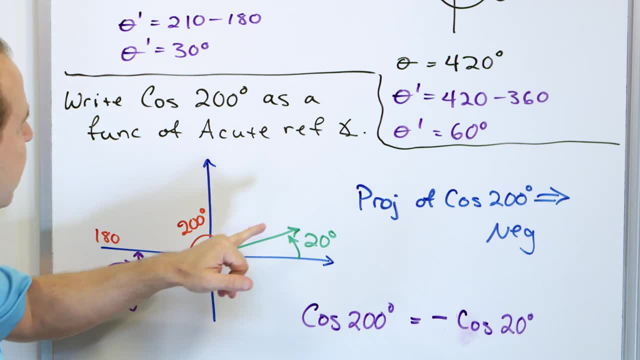 In this case, we go and we say: this is a 20-degree reference angle. So if it were over here, whatever the value of this projection to the cosine, to the x-axis is, whatever it is, we're going to stick a negative on it because the real projection is over here. 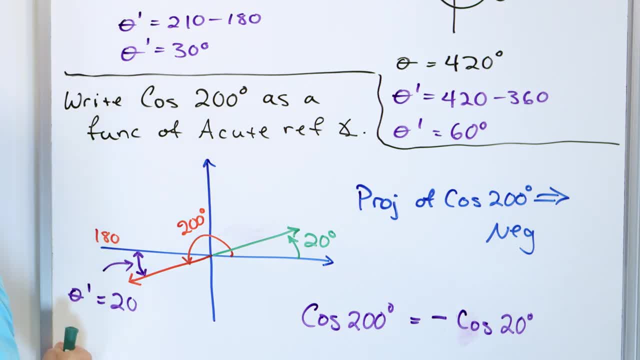 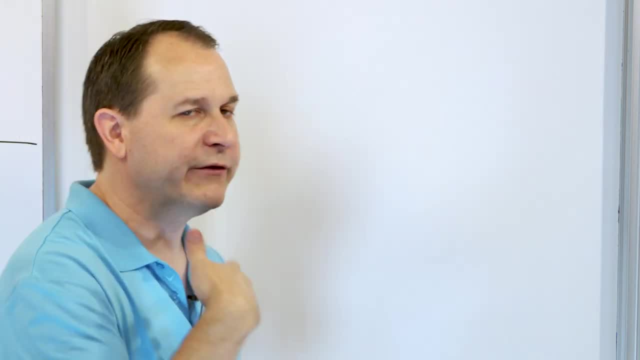 projecting onto this axis over here, Critically, critically important. I encourage you to work the rest of these problems with me And then, as we go on around the unit circle, we're going to do a lot more of this as well. Let's do another one. 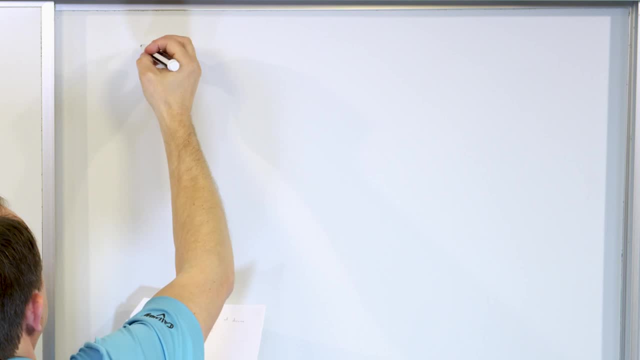 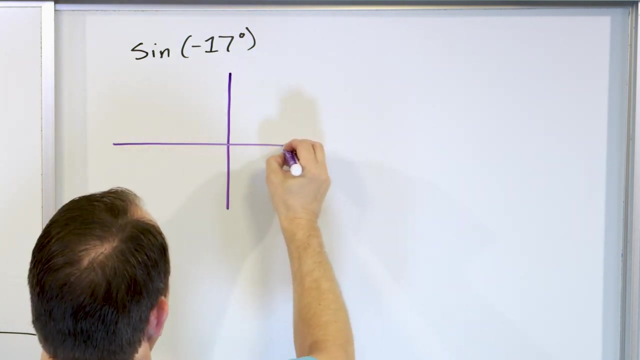 We want to write as a function of an acute angle here, Yeah, of the acute reference angle. What about the sine of negative 17 degrees? The sine of negative 17 degrees? First things first, we must figure out where in the unit circle is this angle. 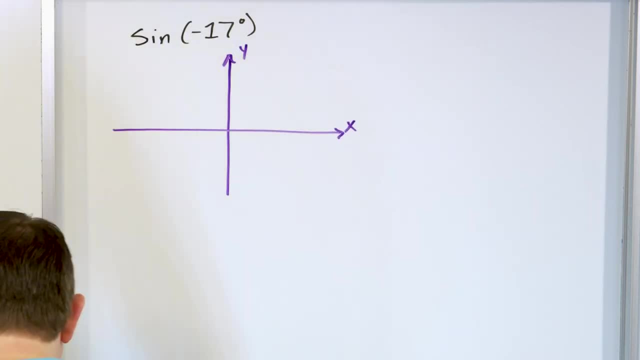 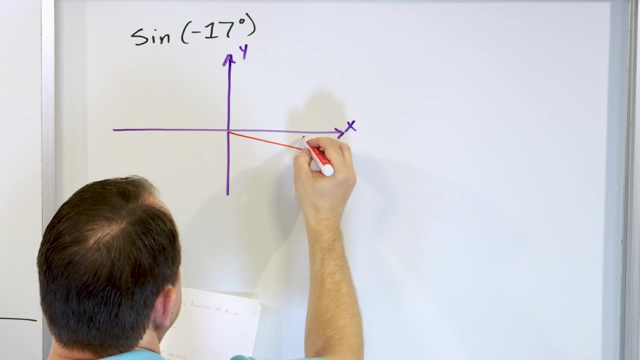 What is the reference angle? Well, it's negative 17 degrees. That means it goes down below the x-axis just a little bit 17 degrees, right? So here, this angle here is negative 17 degrees. That's what that angle is. 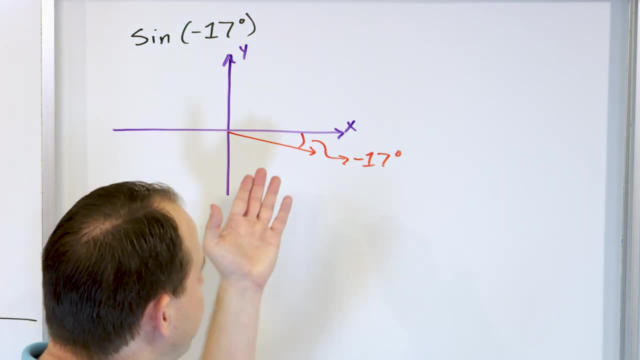 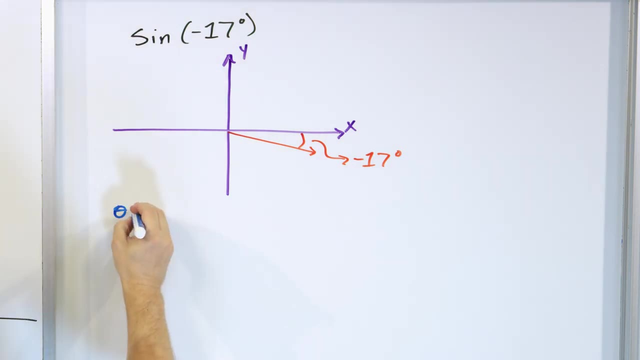 Now, what is the reference angle? The reference angle is the positive acute angle from wherever you are to the x-axis, So the actual reference angle. so we'll say theta is negative 17 degrees, but theta prime is actually positive 17,. whoops, positive 17 degrees. 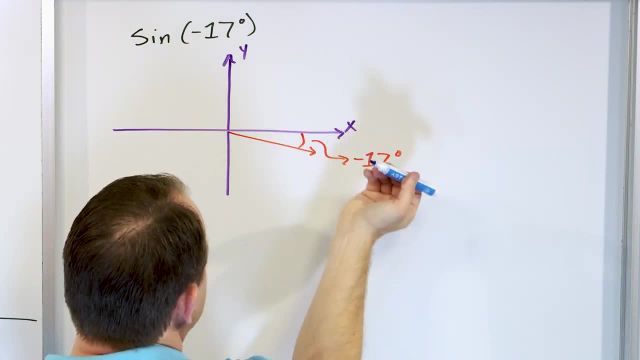 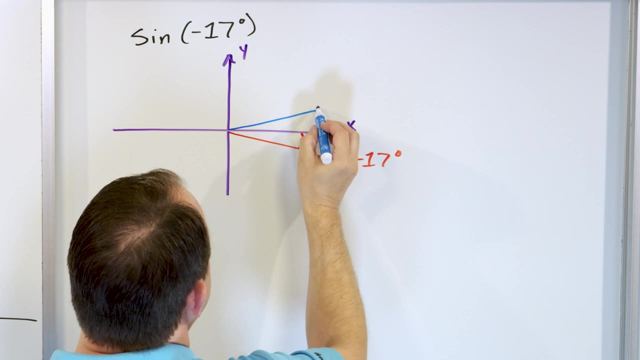 It's just the absolute value of that, because it's just how many degrees are you Like? positive, negative, throw it away. The reference angle is 17 degrees. So if I wanted to draw this reference angle, it would be something like this: 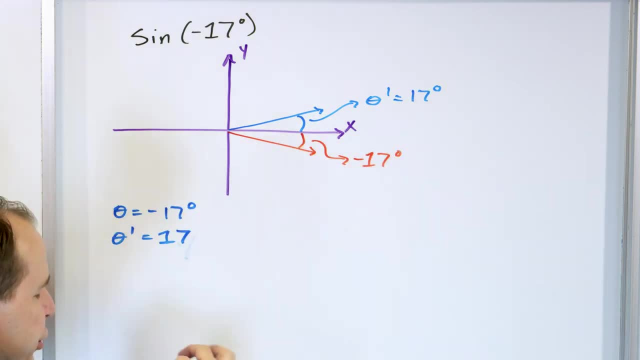 Theta prime is 17 degrees. So basically, you take any value anywhere in the unit circle and you find the reference angle, and then you think about what is the reference angle going to do in quadrant one That's going to give me the value of the sine or the cosine, whatever I'm talking about. 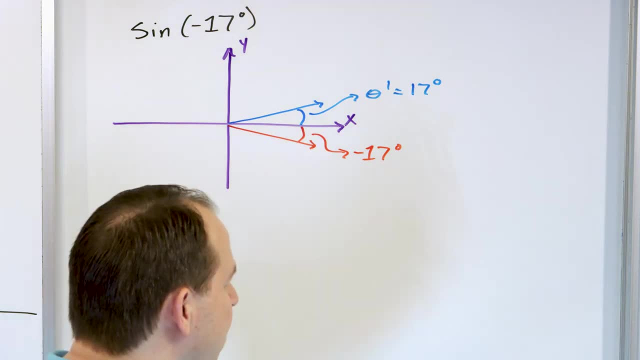 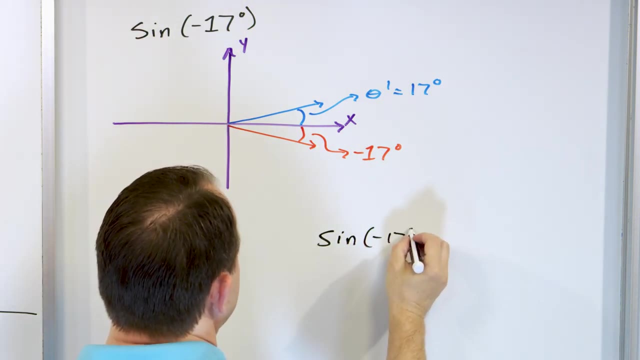 then, to find the value, The value of what I'm really looking for, I just put a sine like a negative or a positive sine on it. So in this case, I want to write this sine of negative 17 degrees is going to be. 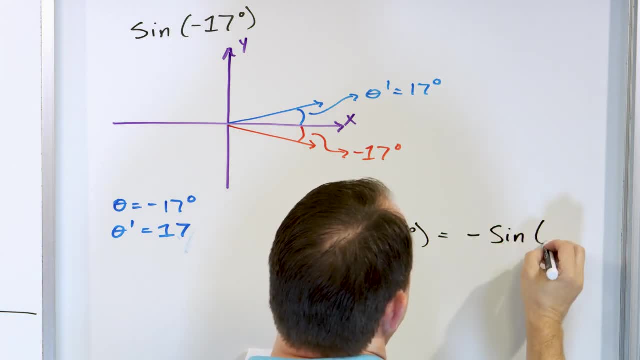 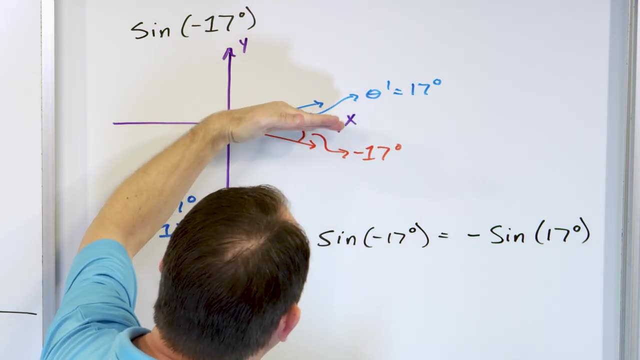 what is it going to be? It's going to be negative sine of positive 17 degrees, In other words, this 17 degree angle that exists up there. it's going to give me some projection onto. in this case I'm gesturing to the x-axis. 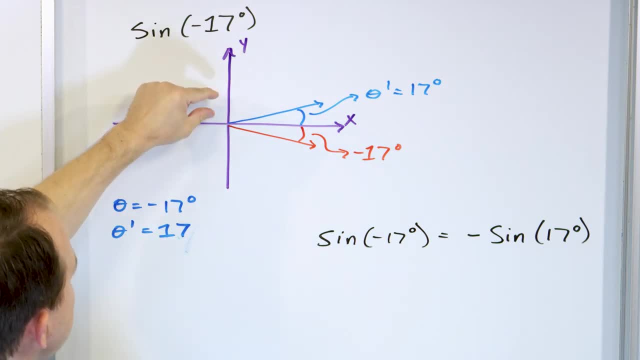 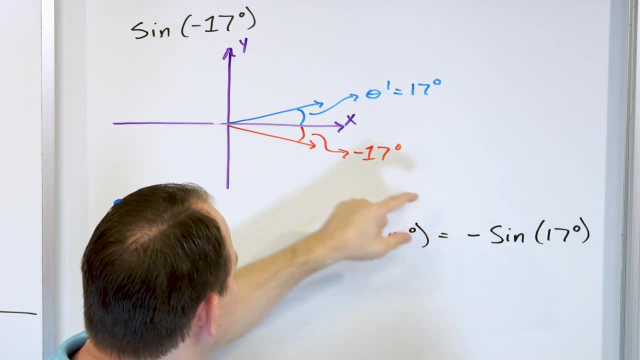 It's actually a sine. So we're getting the projection onto the y-axis here, but this blue line is going to give me a positive projection. Whatever the projection is, whatever answer I get, I slap a negative sign on it and that's going to be the projection of this one. 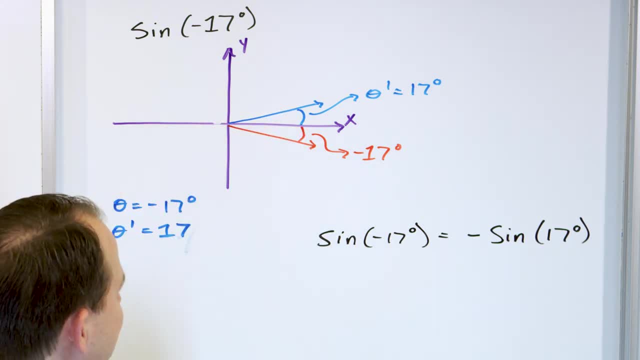 because this one here is really being projected onto the negative axis here. So we're saying that the sine of negative 17 degrees, which is the projection of this guy onto this axis, will give us a negative value. What will it be? It will be the negative of whatever the sine is of that positive angle. 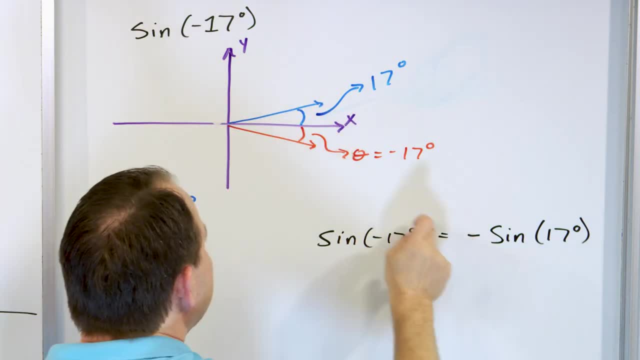 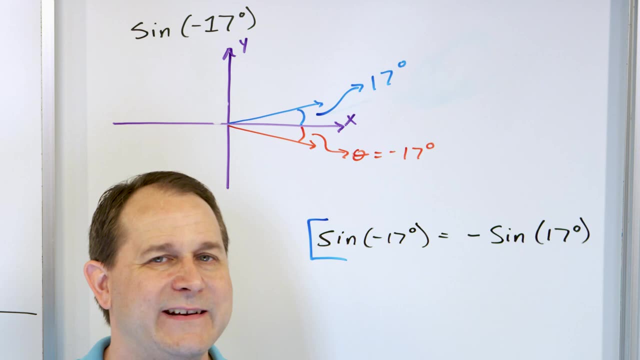 because the projection here gives us a positive value. We slap a negative on it and that's going to give us the projection of what we really are after. So these problems seem crazy- weird, but they're actually exactly what you're going to do when you find 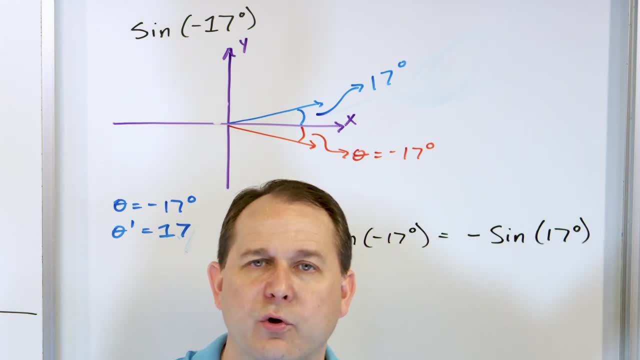 you know what is the sine of 150 degrees on the other side of the unit circle You're going to think about how far is it to the x-axis? figure out what the sine and cosine is and then put a negative or a positive value on it to get the final answer. 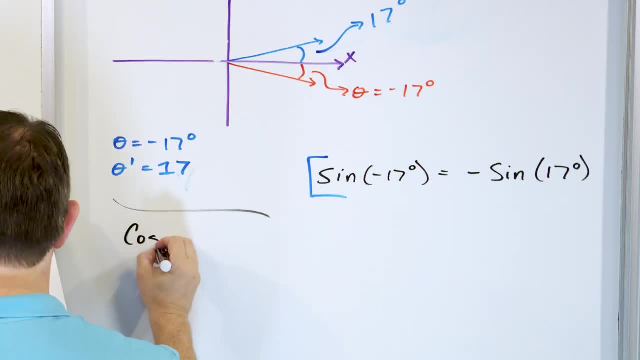 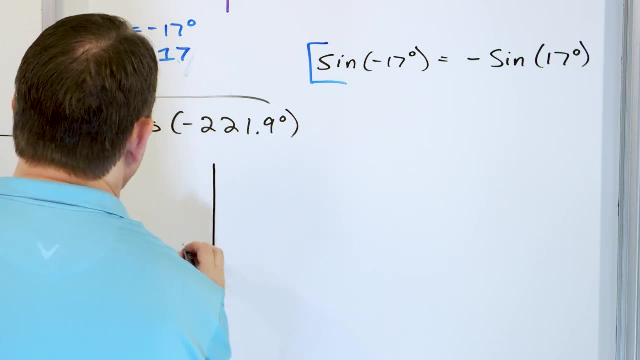 All right, so let's do another one. Let's say we have the cosine of negative 221.9 degrees, like a weird little angle like this: First of all, we need to figure out what quadrant this is in, and we always need to draw a picture to do that properly. 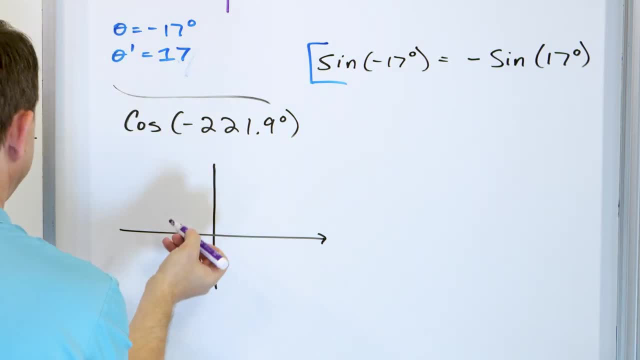 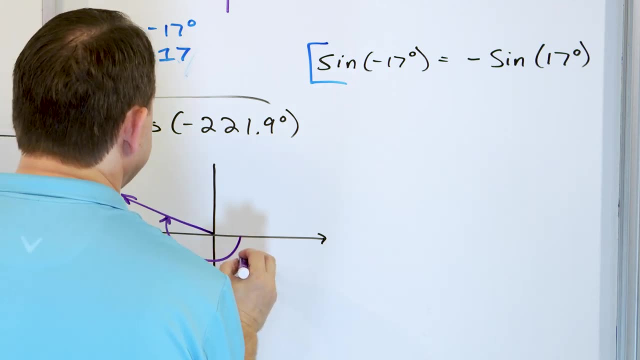 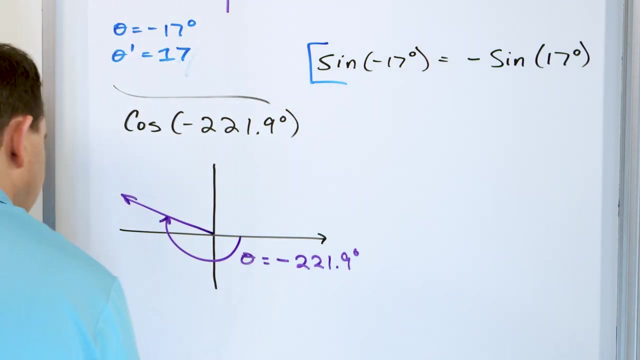 So it's negative 221.. So here's negative 180.. That's negative 270.. So somewhere over here, right, is this angle like this, and so we say theta is negative 221.9 degrees, something like this. All right, So then the question is: what if we? 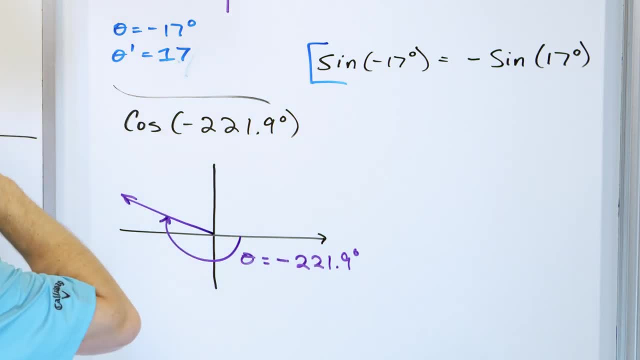 if we want to figure out, if we want to write this in terms of the cosine of another angle, a positive acute angle, then the first thing we have to do is figure out what that positive acute angle is. What's the reference angle? 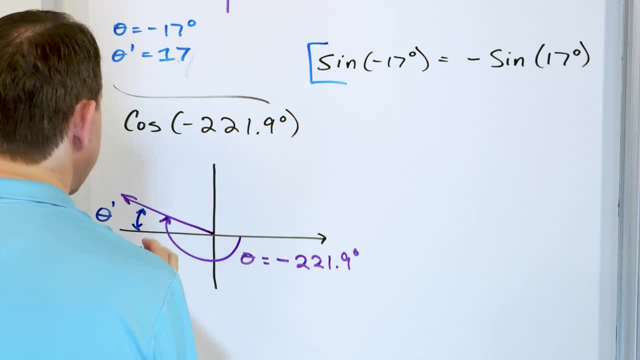 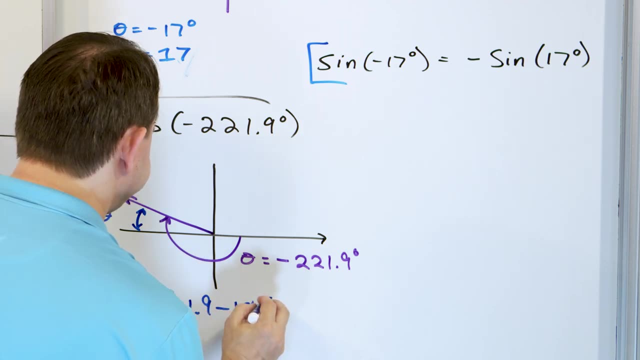 This angle right here is the reference angle, theta prime. So what will it be, Theta prime? Well, let's just take this number: 221.9 minus 180.. And let me make sure I did my math right here: 41.9 degrees. 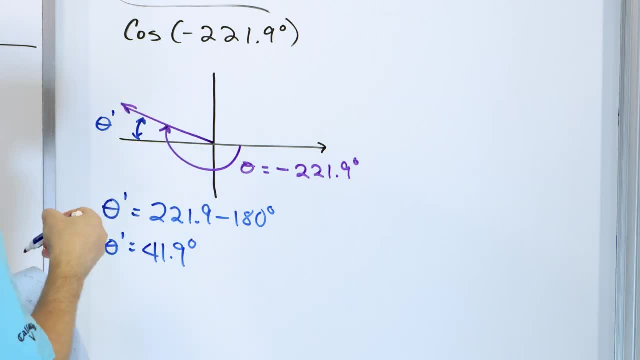 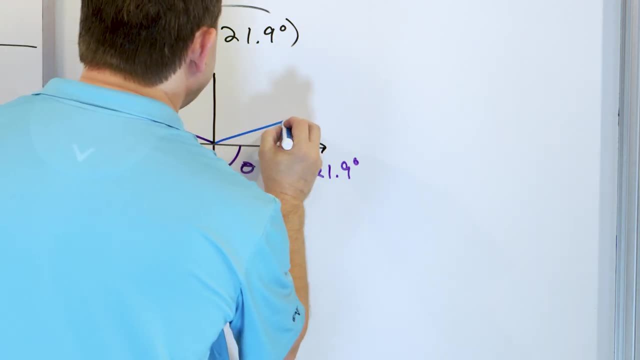 That means if I get a protractor and actually measure this, I get 41.9 degrees. All right, like this. So if I go from symmetry and take a look at it at an equivalent angle over here, that's exactly the same thing. 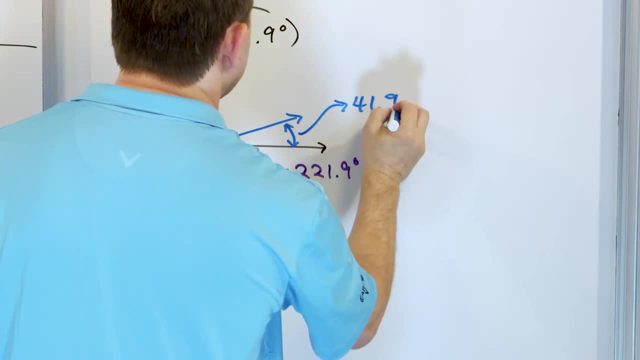 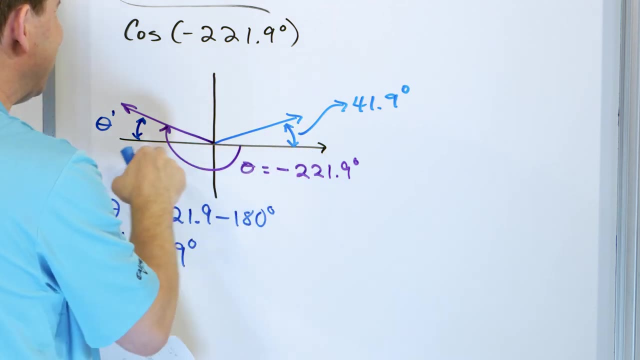 41.9 degrees, like this Right measure to the positive x-axis. If I figure out, whatever the cosine of this angle is, the actual number I get will be the exact same number that I would get over here, but I'd have to stick a negative sign because this is projecting to the negative part of the x-axis over here. 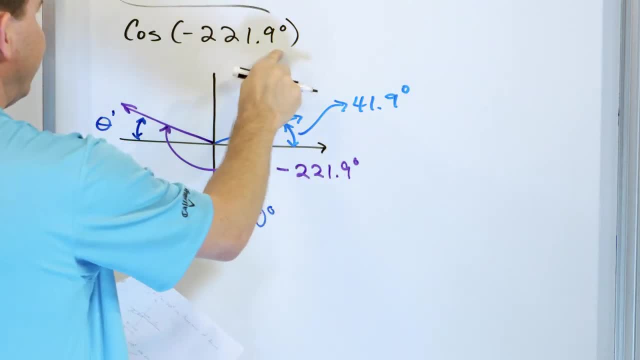 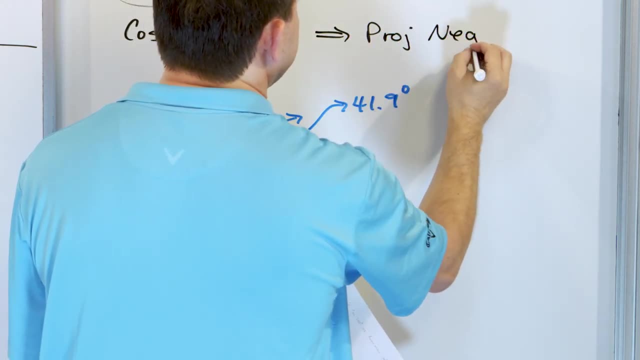 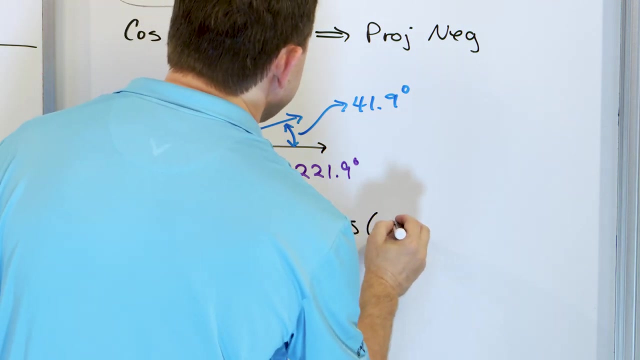 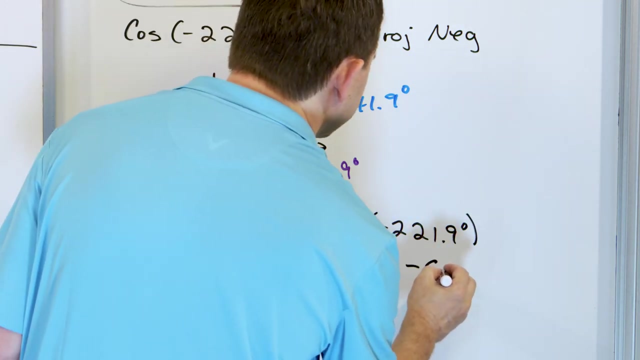 So the bottom line is the cosine of negative 221.9 is going to be projected into the negative axis. So this projection to the cosine here is going to give me a negative number. So because of that, the cosine of negative 221.9 degrees is going to be equal to the negative of the cosine of 41.9 degrees. 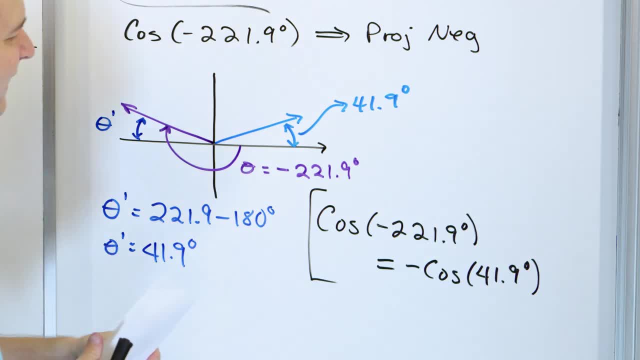 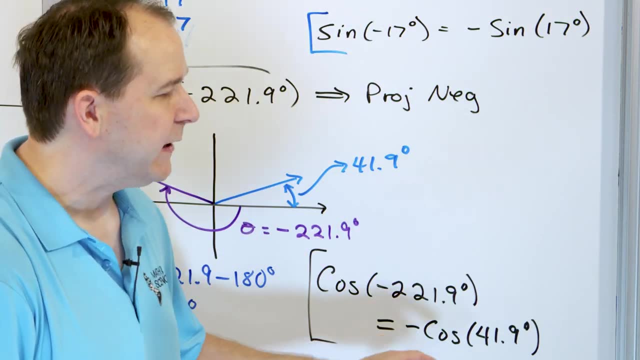 Negative of cosine of 41.9 degrees. So I encourage you to do this: get a calculator, put 41.9 degrees, Make sure you're in degree mode, hit the cosine button and slap a negative on it and figure out what answer you get. 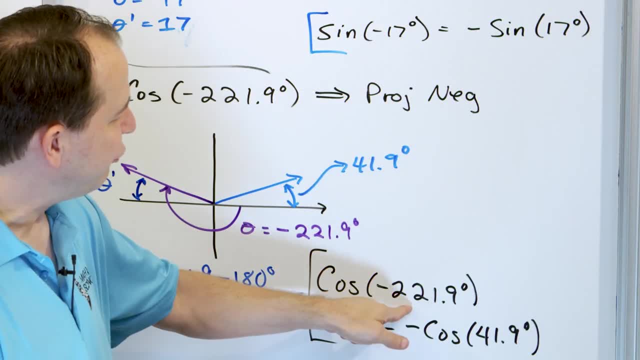 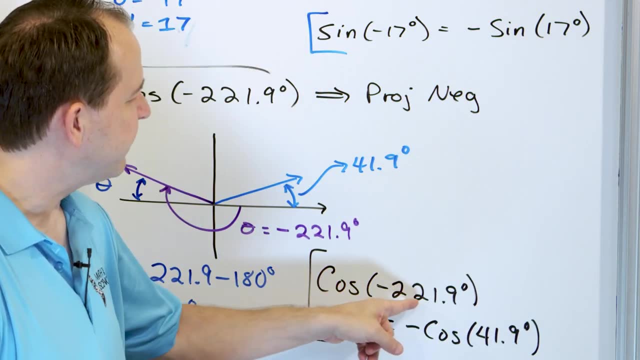 You're going to get some number, then separately put negative 221.9 in the calculator, hit the cosine button. Those two numbers will be the same. if you're trying to figure out what the cosine of this negative angle is, What we always do in trigonometry is we say: well, 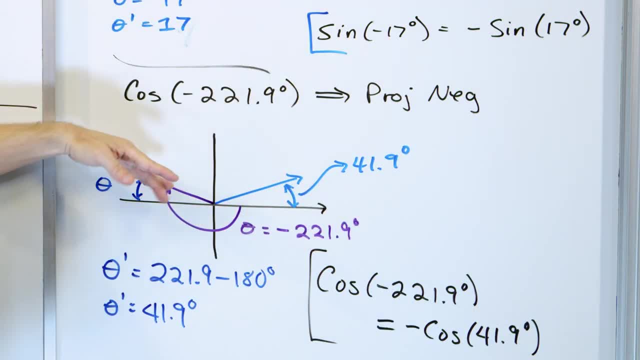 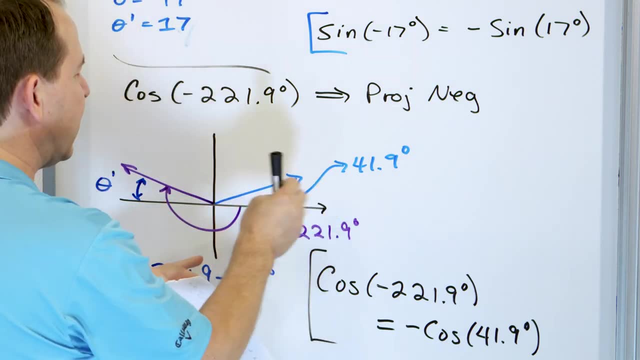 first of all, what is the angle, even though I know it's way over here? What is the angle between this And the positive and whatever the closest axis is? then I pretend that that angle is over here and I figure out what the cosine is. and then, whatever number I get, I just slap a negative. 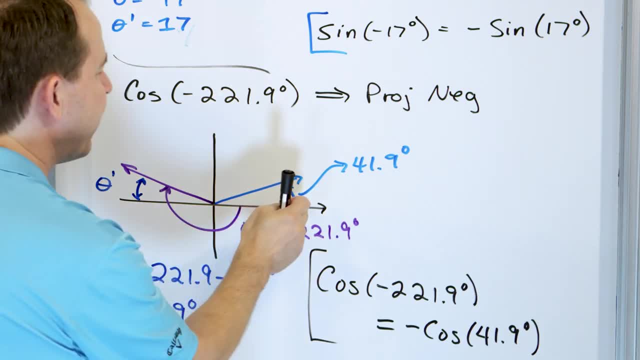 or a positive value. in this case, the cosine is negative. So whatever value I get here, I'll just have to put a negative sign on the on the output of it, because this is always going to project to a positive cosine over here. So again, walking it back to the unit circle. 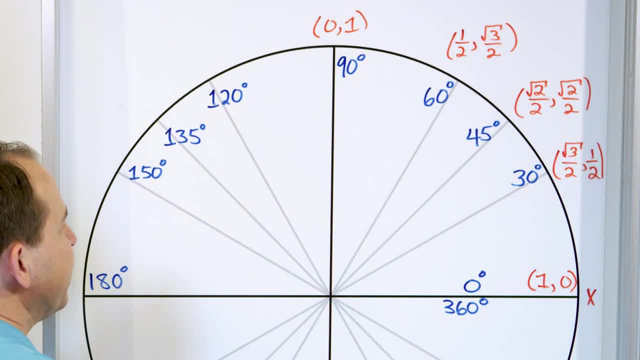 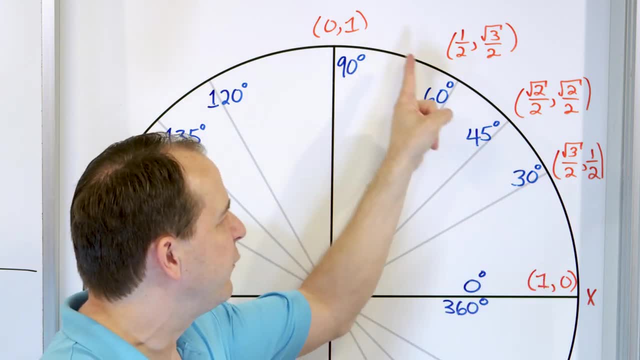 We know what the signs and the cosines are of all these angles. So essentially, the values of the cosines and the cosine Of all the angles all the way around the unit circle will be the exact same numbers as the ones we have here. 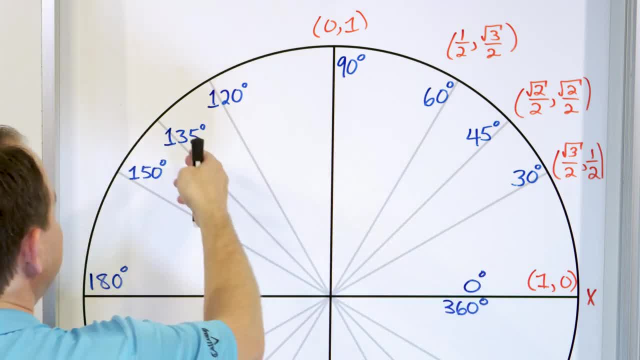 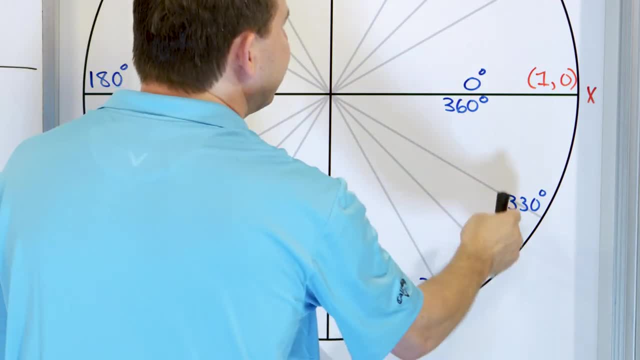 It makes sense. The projection here should be the same as the projection here, forgetting about the sign of the positive or negative. same as the projection here. same as the projection here, because the angles are all the same to the x-axis. It's just some of these project to positive x-axis. 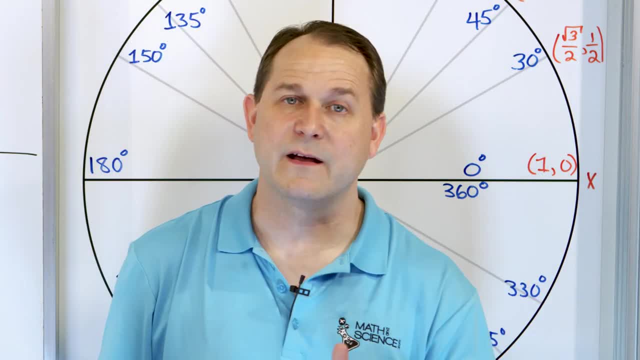 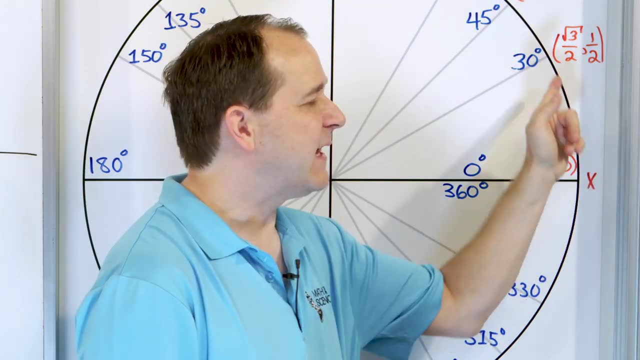 and some projected negative, and some of them projected a positive y-axis and some projected negative at the y-axis. So by looking at what reference angle we're at, then we can figure out what the sine and cosine is as far as the number goes, and then we can just stick a negative or a positive sign on it. 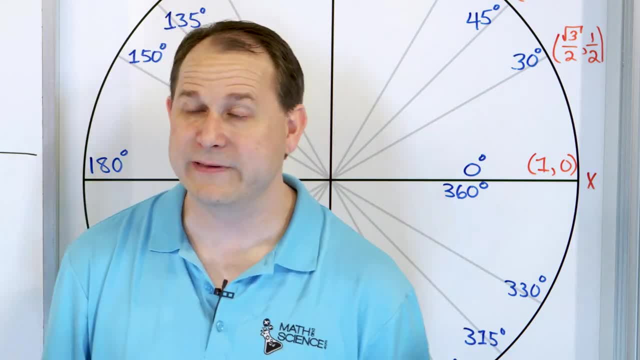 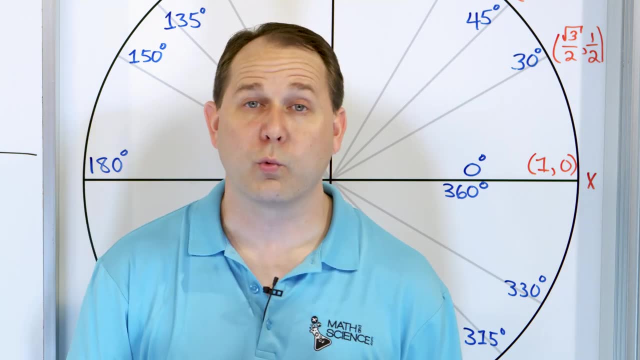 depending on what quadrant we're in. We're going to be doing a lot more with this. This was just the introduction to it, So for now, I want you to kind of try to get the idea here. Make sure you understand this. We're going to do more work with reference angles in the next section. 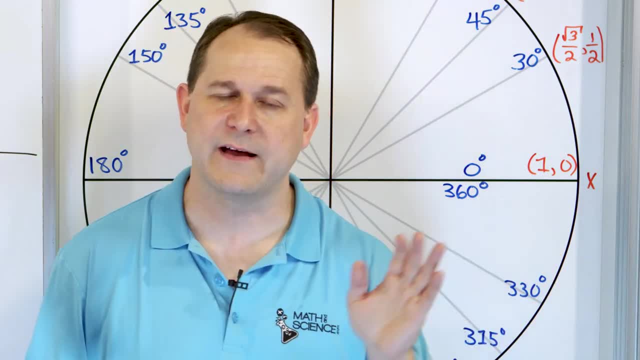 and then we will be going all the way around the unit circle and filling out all of the signs and cosines for all of these angles.